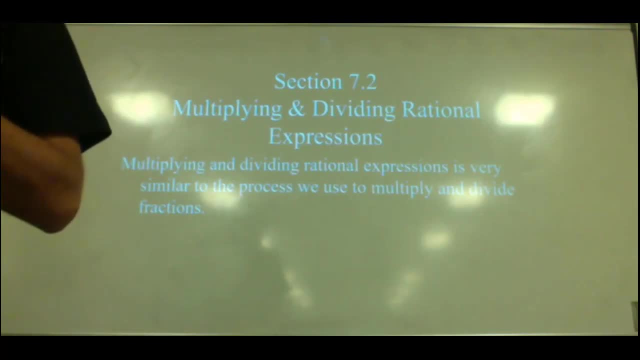 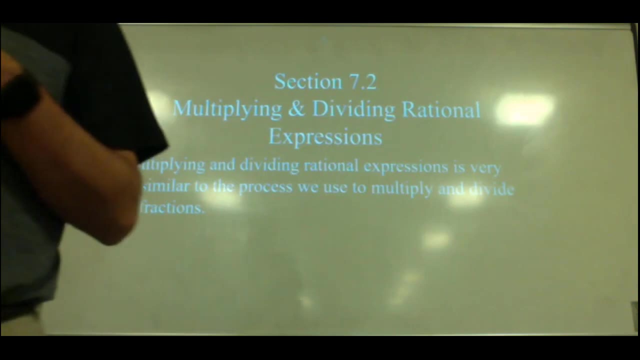 Same exact problem. Well, I mean not as many, but it's not going to be every problem- from your test. I mean I suppose I could do that, but that would be like seven tests, That would be rough. But anyway, all the problems on the final you will have seen before. Okay, Cause they will have. 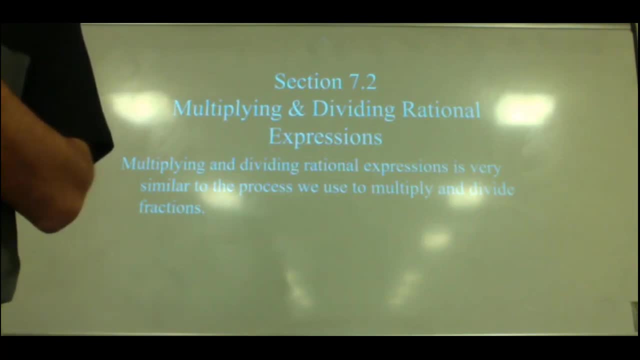 been problems from your test, But obviously that's eight chapters worth of stuff, So it's not like it's going to be super easy. but also, reviewing your test is going to help you in preparation for your final too. So you make sure, cause I'm not throwing anything new on the final. 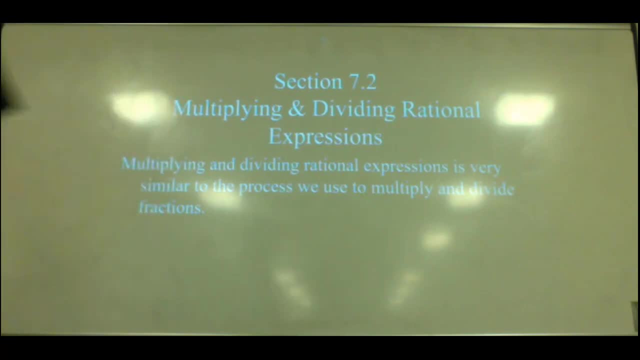 It's all stuff that we've done already and that we've tested over. Okay, All right, Let's continue with section seven. Uh, two, if you remember section seven one, we were simplifying these rational expressions And when we simplified, remember we would try to factor And then, if there were any factors in the 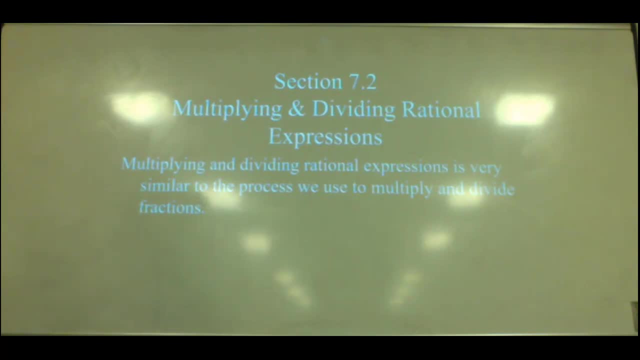 numerator and the denominator that were the same, we were able to cancel those factors and they would become ones. Okay, Today or tonight. in section seven two, we're moving on and we are multiplying and dividing the rational expressions And you'll find out, multiplying is really. 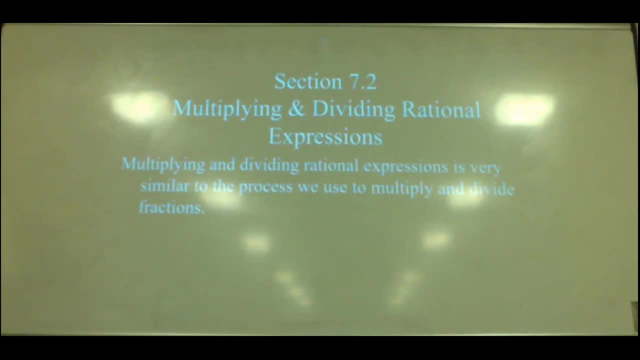 really similar to what we did last Week. dividing is really similar, but there's one extra step. Okay. So multiplying and dividing rational expressions is very similar to the process that we use to multiply and divide fractions, Because these aren't fractions, They're just not fractions. 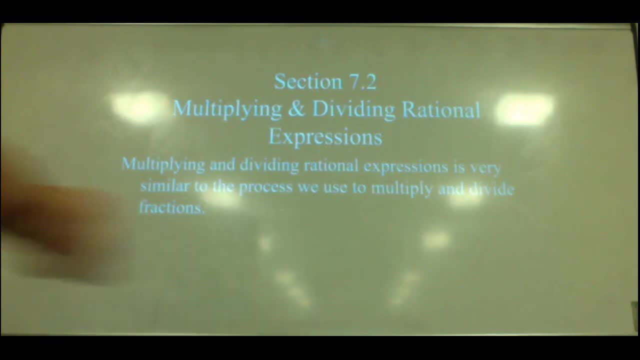 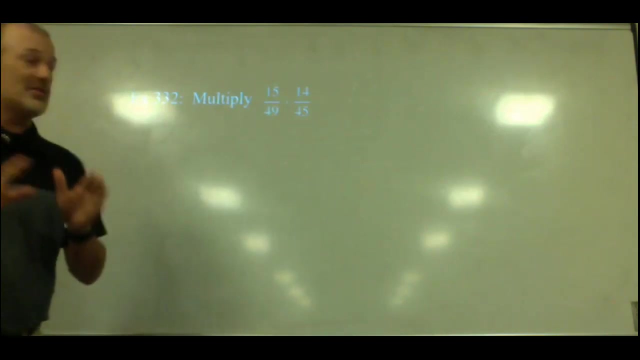 of like just numbers. they have the variables in them. Okay, so we're going to take a look at turning the science so that it works. And so let's just remind ourselves if we multiply fractions. Now, typically They say what you guys- and I understand this, I totally understand- but typically what you would do if 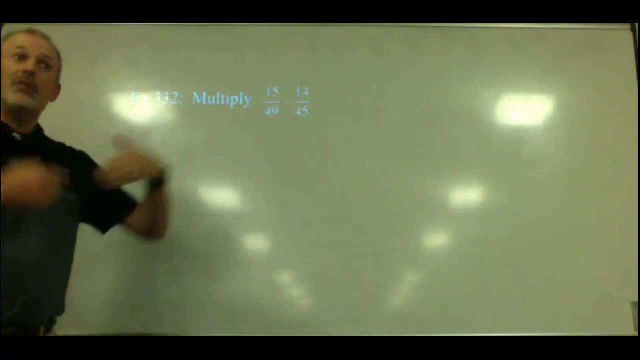 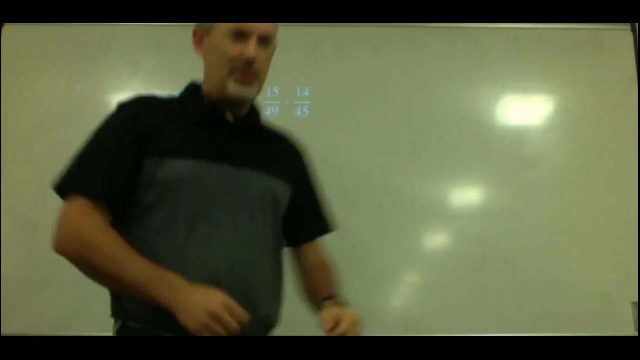 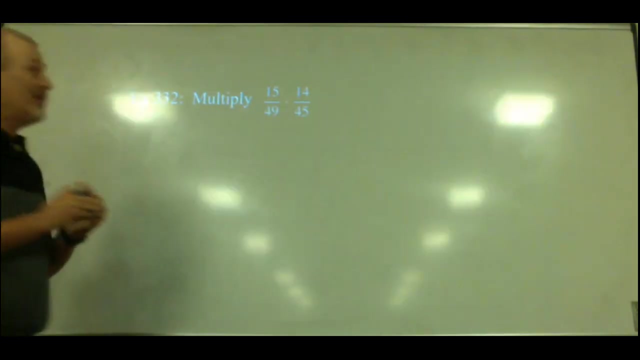 you're multiplying these is. you probably just type it into your calculator. But I want us to think about what's actually going on here in preparation for what we're going to do tonight. So if we take the 15, and let's take the 15 and let's break it up, let's factor it into its prime factors. 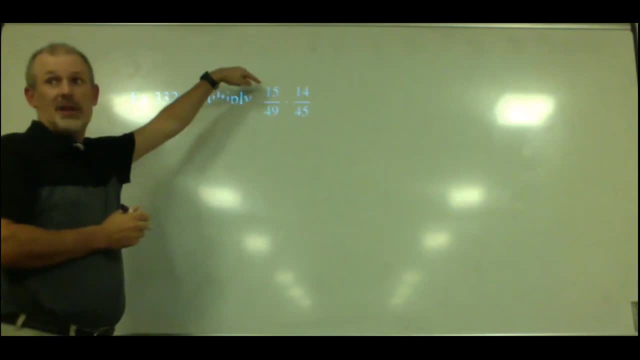 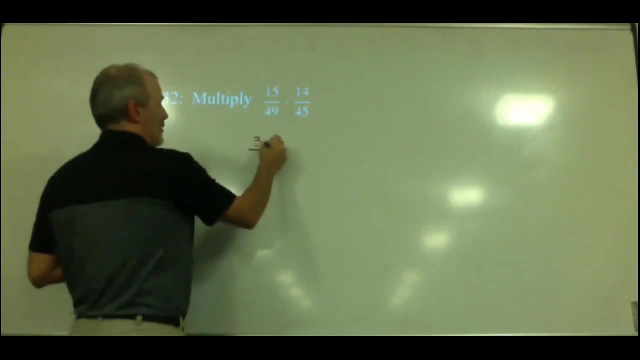 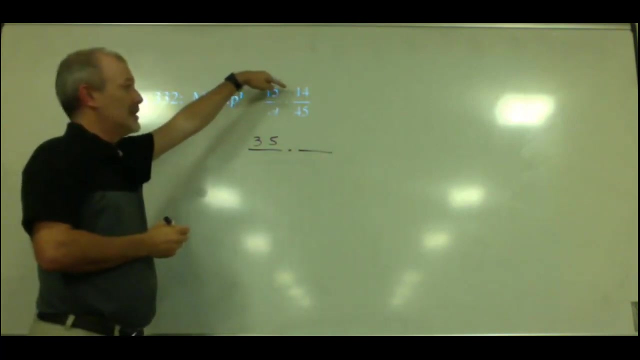 How can we break up 15? Five times, excuse me, five times three. So 15 is- and I'm going to put it in order here- three times five. And then 14- is what times what? Seven, Seven times two, Okay. 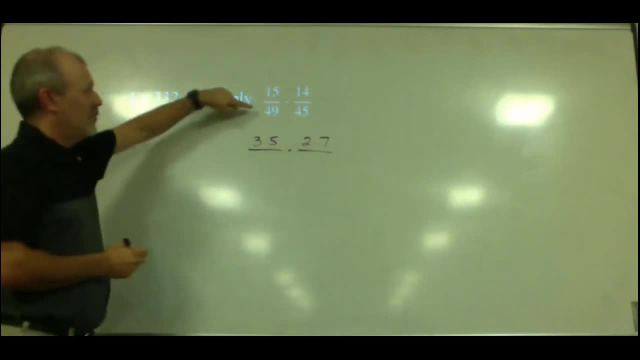 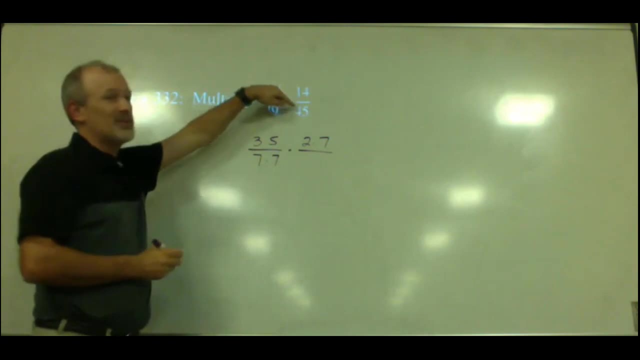 so two times seven, Okay. and then 49- is what times what? Seven times seven, And then 45,. this one's tricky because it's It has three, it's nine, but nine can break up into three and three again. 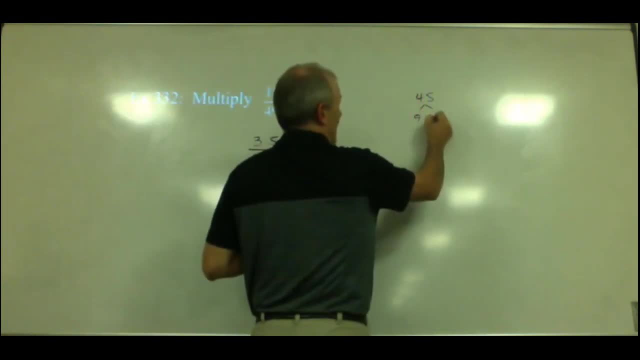 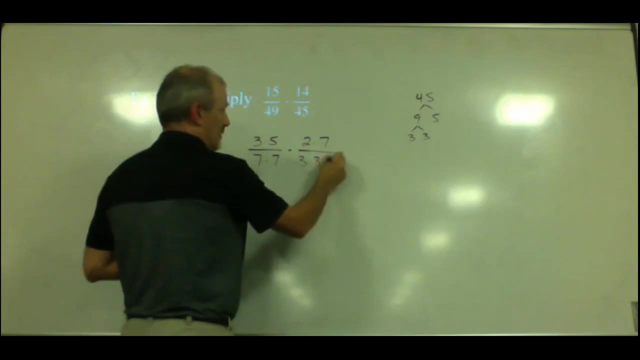 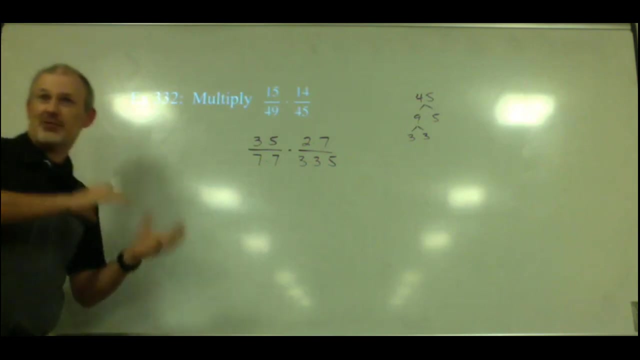 So we'll do that. one on the side 45 breaks up into nine times five, but nine can break up into three times three, So it's three times three times five. Okay, Now when we multiply fractions again, this is actually all the way back to chapter zero. 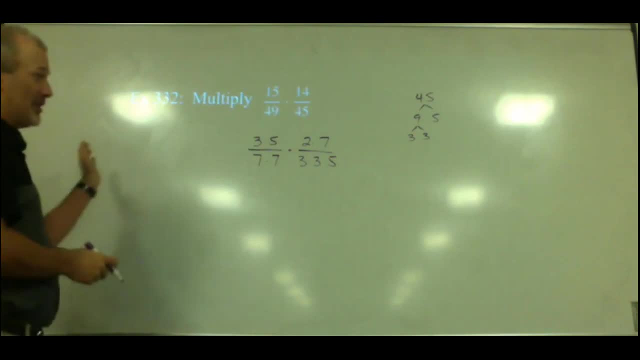 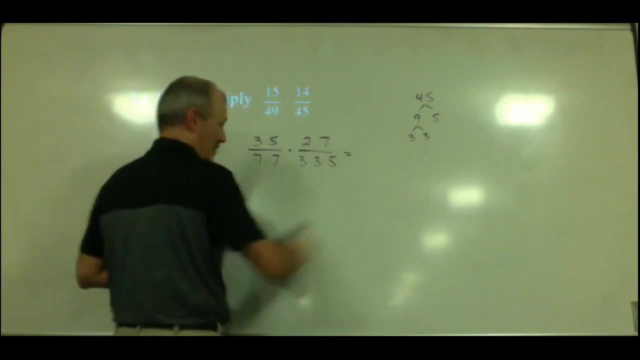 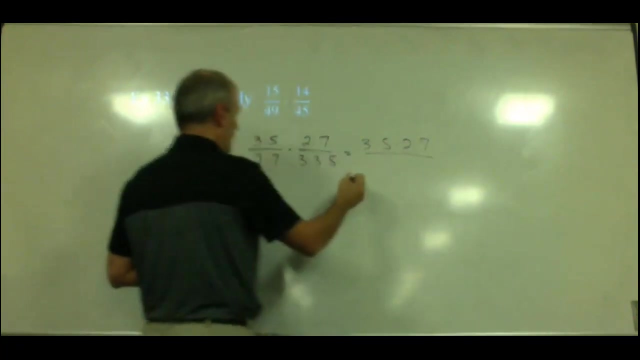 that we did that very, very first night. We multiply straight across. So what we will have if we multiply straight across is- and I'm just gonna, I wanna leave it this way so that you can see it- You've got three times, five times, two times seven. 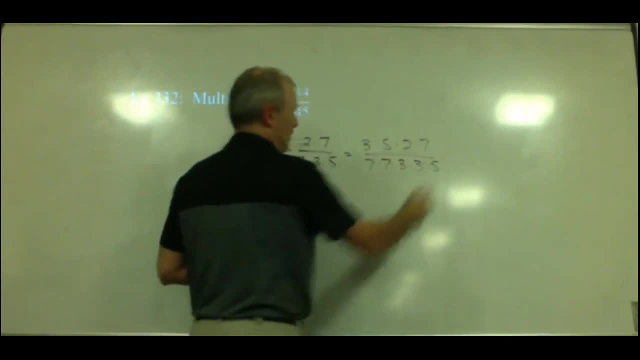 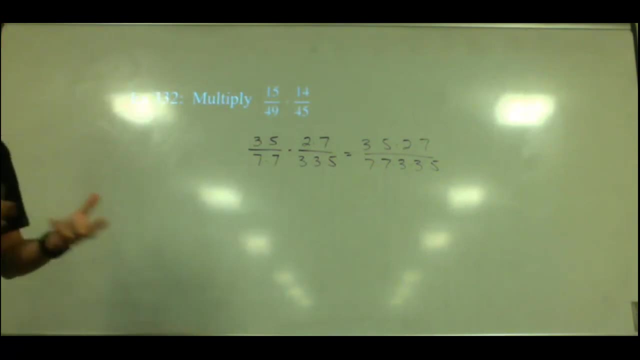 over seven times seven times three times three times five. Right, you, just you put it all together: The top stays on the top, the bottom stays on the bottom, but now it's one big fraction, Okay, And once we have it written like this: 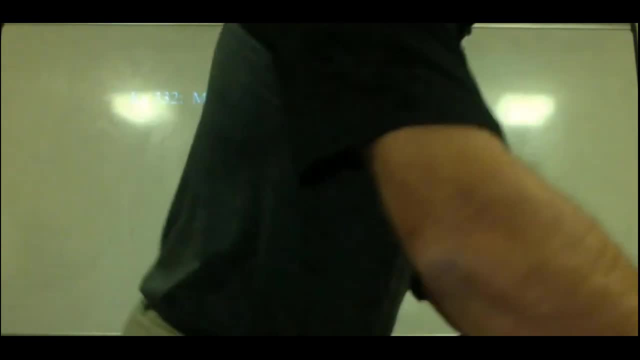 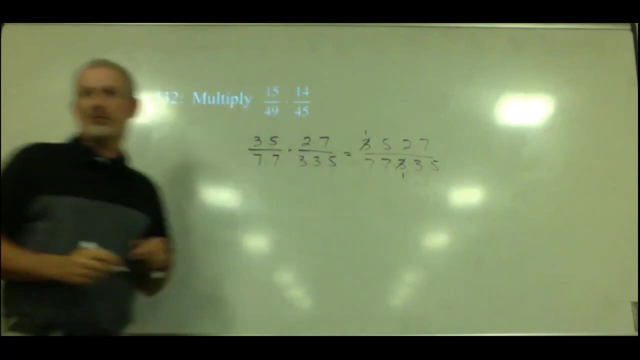 anything that's in common can be canceled out, And so notice, we have a three up here in the numerator that can cancel out with one of the threes in the denominator, not with both of them, but with one of them. We also have a five up here. 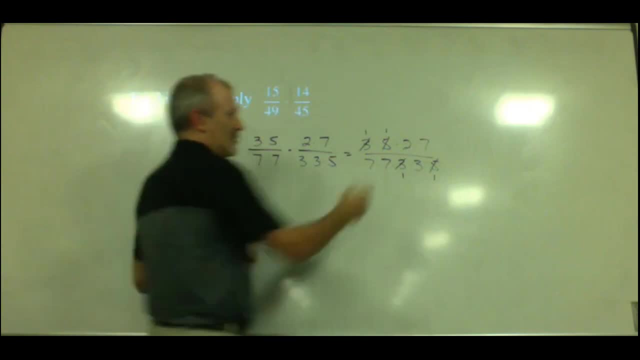 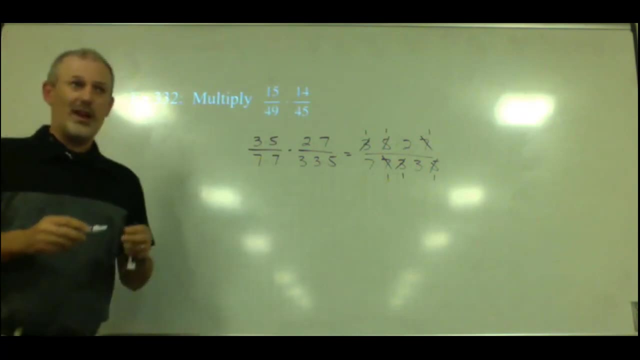 that can cancel out with five down here. We also have a seven up here that can cancel with the seven down here, And so notice all that we have left. besides the ones, because multiplying by one doesn't do anything- All we have left on the top is two. 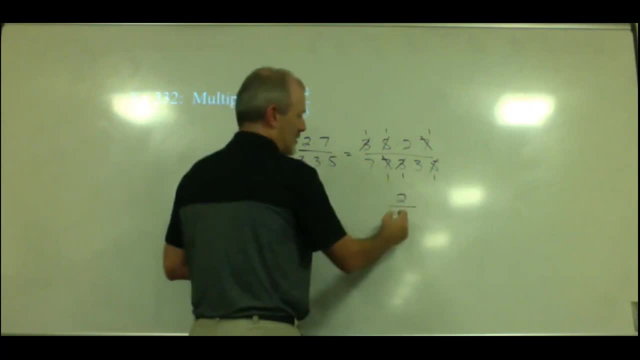 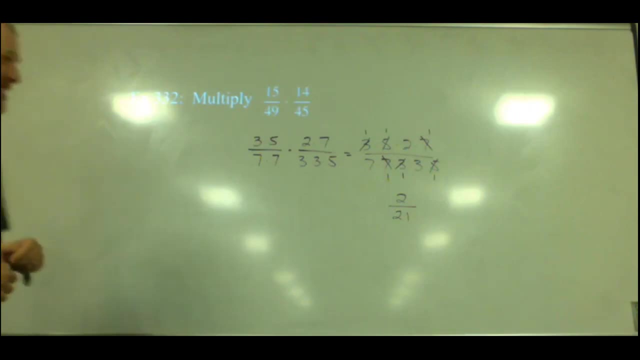 And what we have left is two, And what we have left on the bottom is seven times three, which is 21.. So that would be our answer if we multiplied that all together. Now, the reason I do that is because I want to illustrate something. 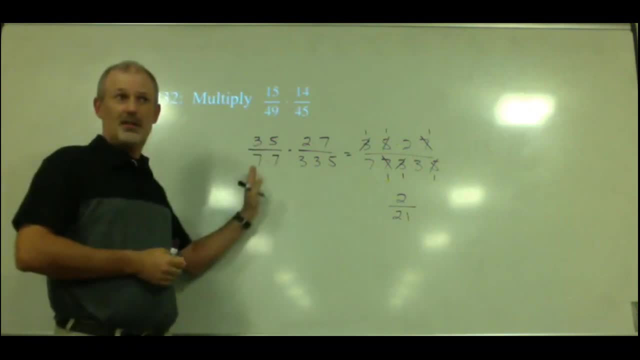 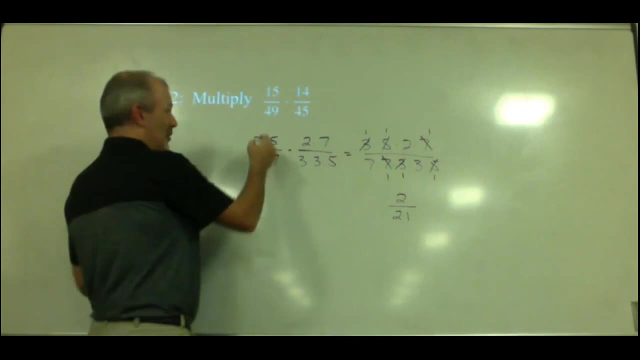 Notice that when we see it like this, written like this, we don't have to rewrite it again, all as one fraction, because we know that's what's going to happen. So we could cancel this three right here, and we could cancel this five right here. 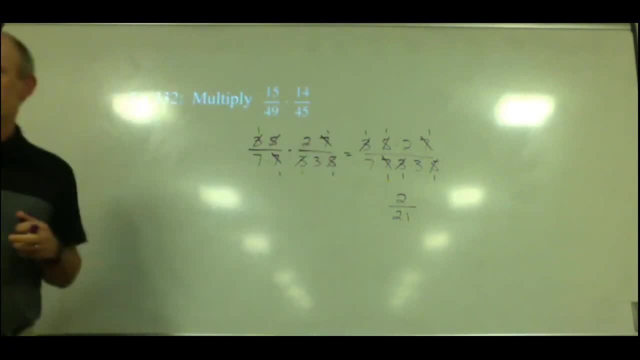 and we could cancel this seven right here and it would do the exact same thing, Right? So when we're canceling, as long as we're canceling from the numerator to the denominator, it doesn't matter which fraction we're canceling in. 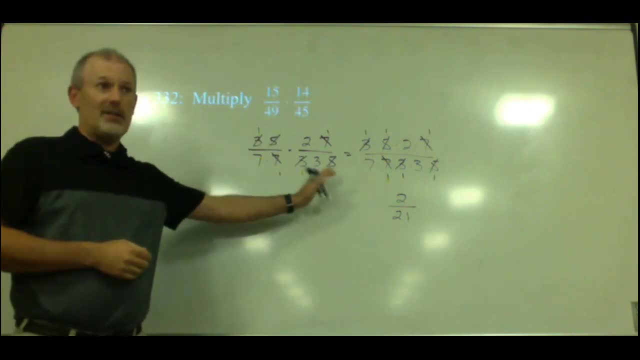 So it can be the first numerator with the second denominator, that's fine, Or the second numerator with the first denominator, because again, when you multiply, it just all goes together as one fraction anyway. Okay, Now, if that's confusing, don't worry about it. 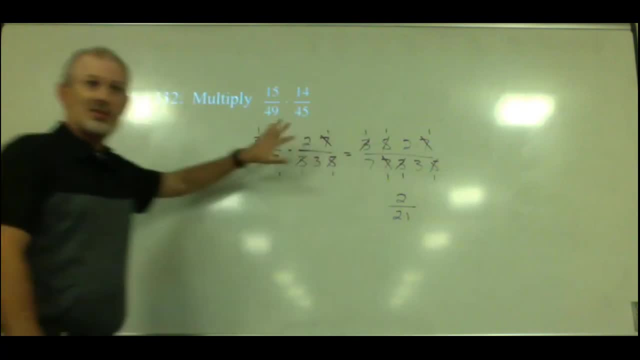 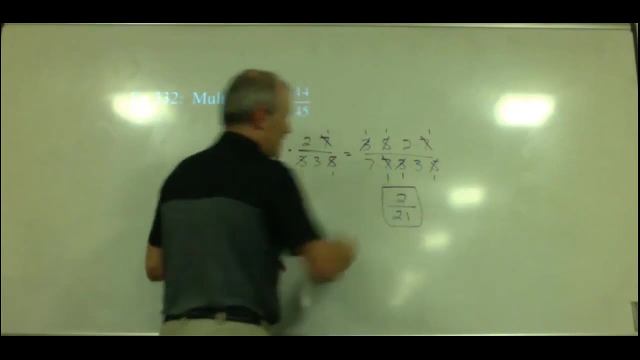 Just write it all as one fraction and then do your canceling. But this is just to save you a little bit of time. But two over 21 would be our answer there after we cancel. And you can see after you cancel. the numbers are really easy to multiply. 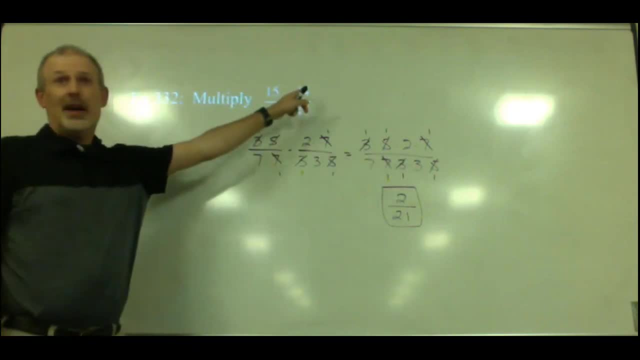 Whereas if I was multiplying 15 times 14, I don't know that in my head. Or if I was multiplying 49 times 45, I don't know that in my head, But once you cancel, then the numbers are much smaller. 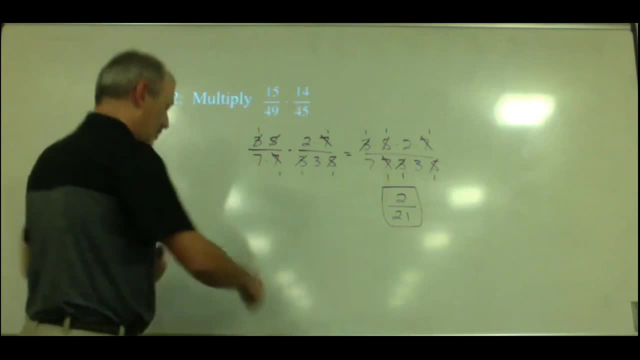 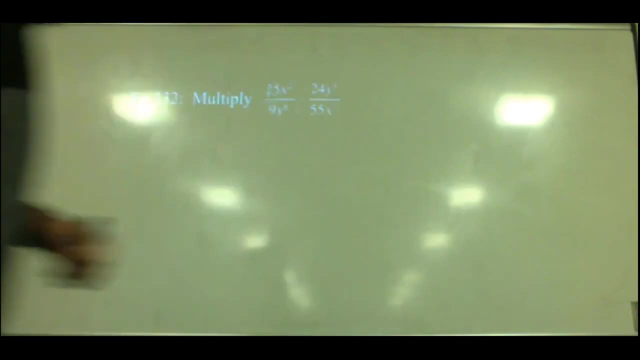 much easier to work with, And that will be the case for our polynomials as well. So, Okay, Let's go ahead and look at this one. So this one. we've got numbers again, but we've also got variables. Okay, 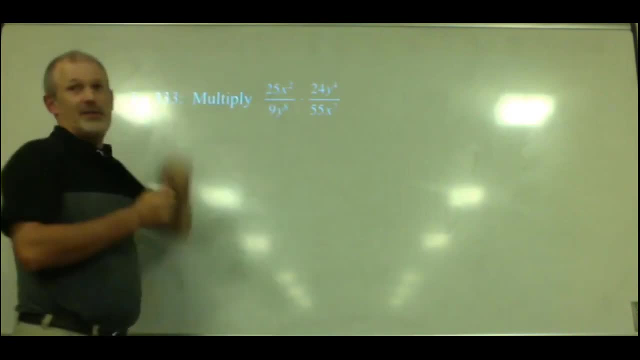 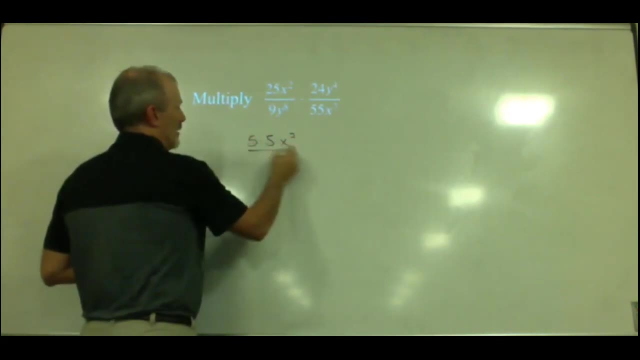 So let's do the same thing. How can we break up the 25? Five times five, And we know we've got an X squared there, And on the bottom we've got nine Y to the eighth, which would be three times three Y to the eighth. 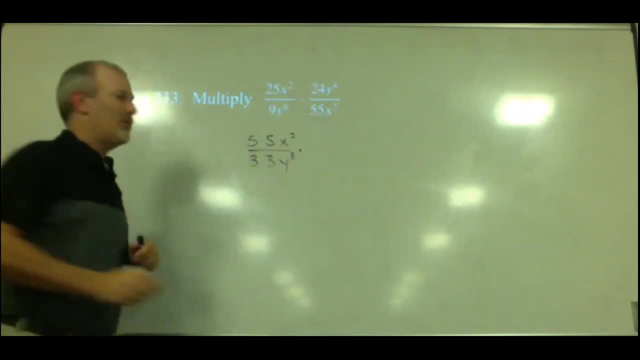 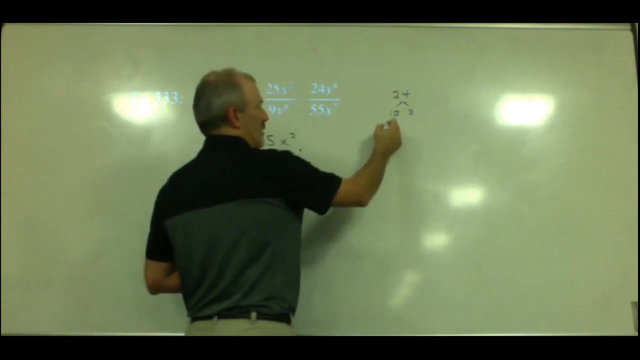 And then times. How can we break up the 24? That one again has more than just two factors. How could we break that up? Well, 12 times two, And then this could be break up into three. I think you're giving me. 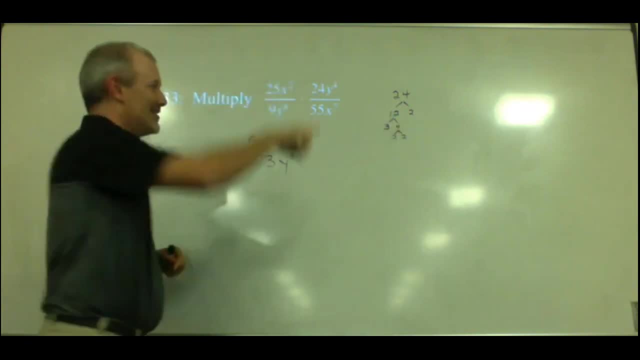 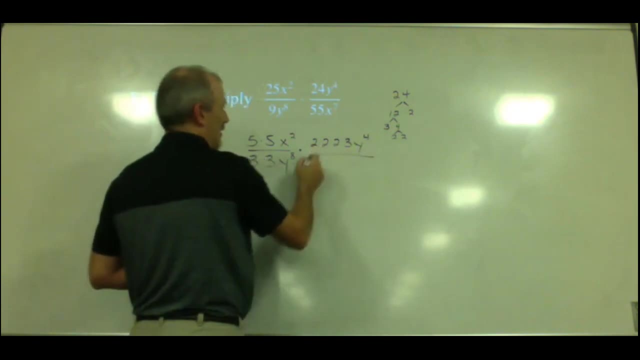 so three and four, and then two and two. right, So it's all the ends. Three times two times two times two. So two times two times two times three, And then Y to the fourth, And then here 55. That is five times 11 and X to the seventh. 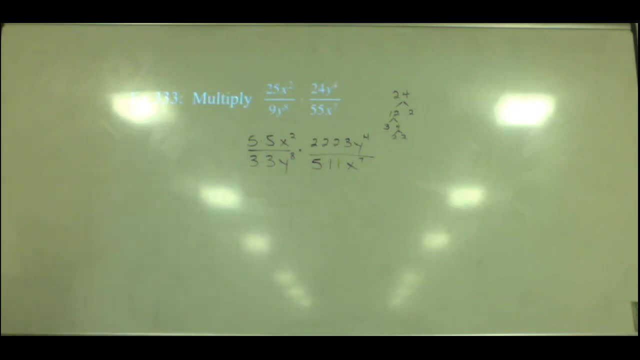 So let's see, let's start with the numbers, because we just did an example like that- Are there any numbers that we can cancel top to bottom? Five, Five, Okay. So let's cancel out this five with this five and they become ones. 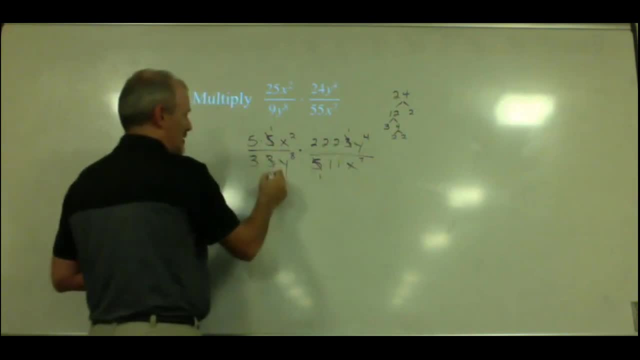 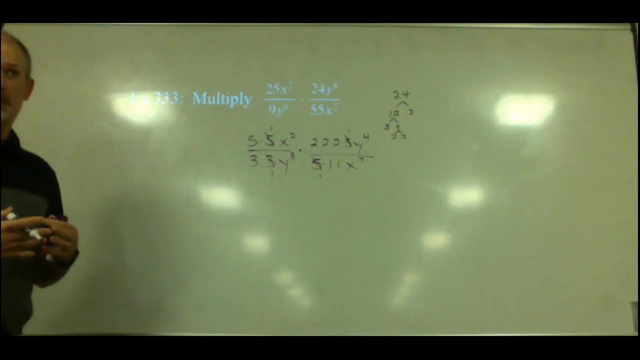 And then, yes, I heard a three, And so we can cancel that three with one of these threes And those become ones. And that's all as far as the numbers that can cancel out. Does that make sense? All the other numbers from top to bottom: 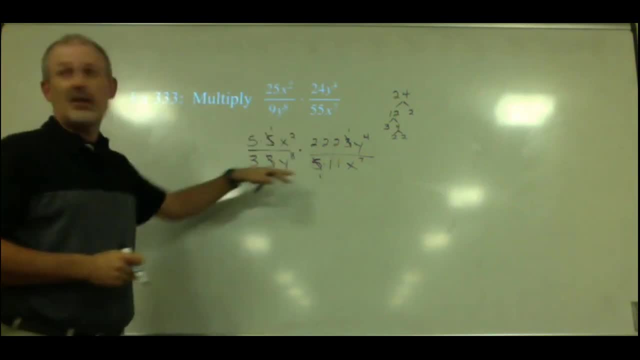 There's a five here, but no more fives down here. There's twos up here, but no more twos down here. So then we just multiply all those numbers back together Five times two times two times two, And if you want to use a calculator, that's fine. 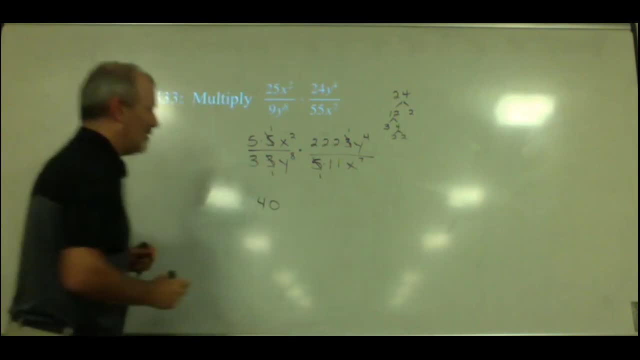 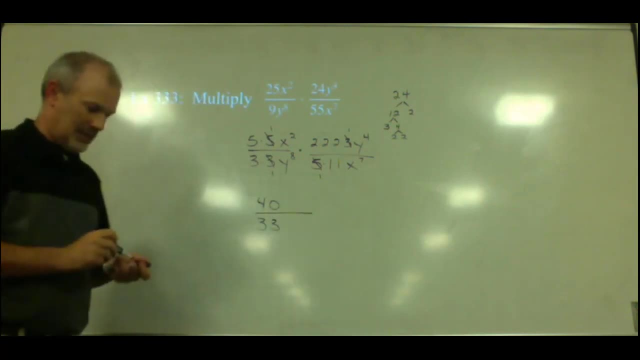 It ends up being 40. on the top- I guess I'm using black now- And on the bottom, three times 11 is 33.. Okay, So that's the number part. Now we also want to look at the variables, And if you remember, we did these in chapter five, I think. 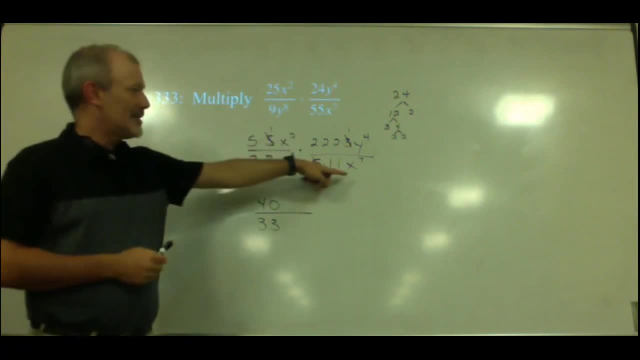 So we've got x squared on the top and x to the seventh on the bottom. What happens with those two Subtract? Yeah, you subtract- And I always do- the bigger one minus the smaller one. So seven minus two is five And it ends up being on the bottom. 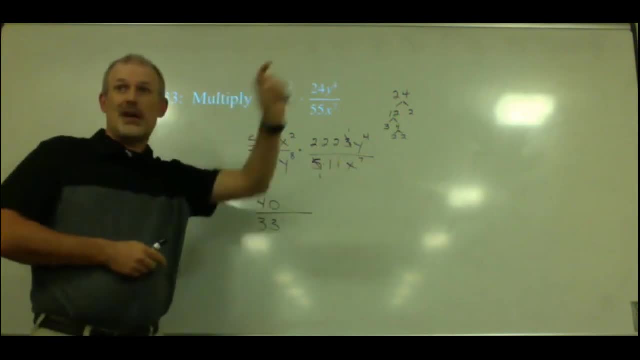 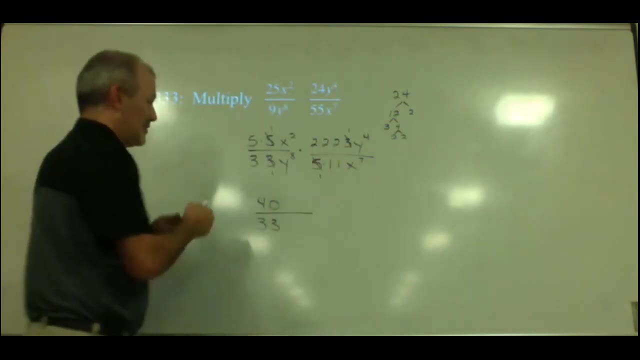 because that's where the bigger one is. So it's like you have two x's on the top and you have seven on the bottom. So when you cancel there's still five left on the bottom. So x to the fifth goes on the bottom. 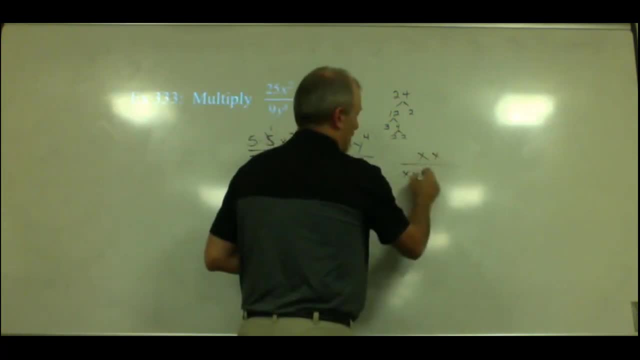 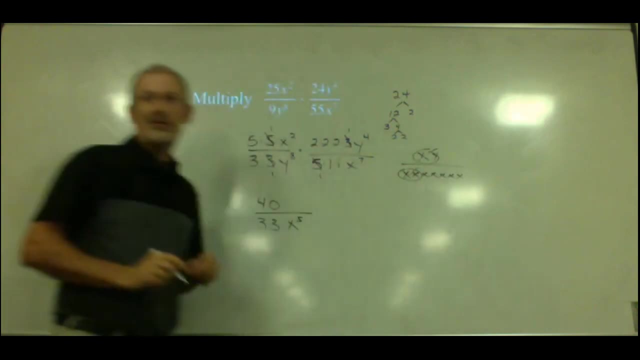 And if you need to draw that out, you certainly can. There's x squared And there's x to the seventh. These two would cancel with those two And you still have five left on the bottom. Okay, if you want to draw it out, you certainly can. 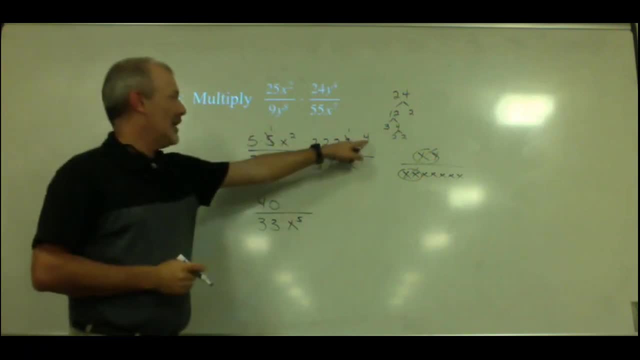 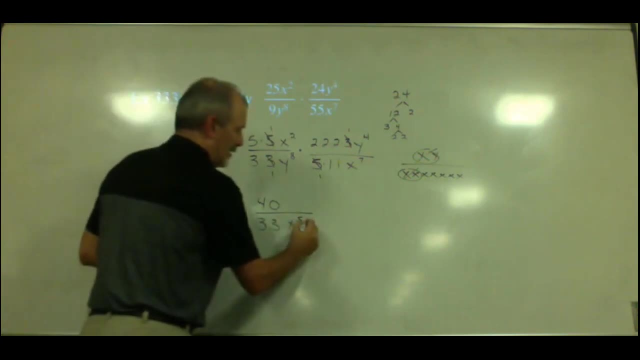 So that takes care of the x's. And what about the y's? You've got y to the fourth on the top and y to the eighth on the bottom In the denominator Y to the fourth, Y to the fourth, And that will be in the denominator. 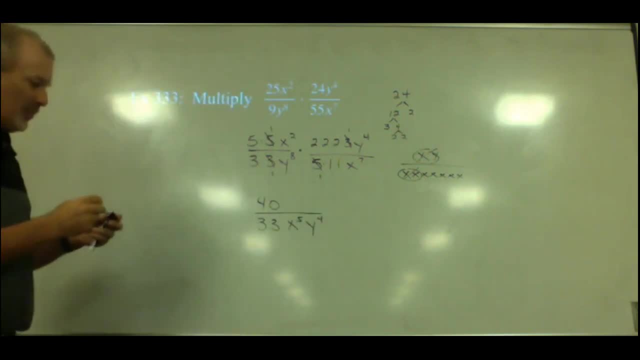 That's right, And so that's our answer: 40 over 33x to the fifth, y to the fourth. So that first example we did in chapter zero. This example we did problems like this in chapter five. Okay, we may not remember. 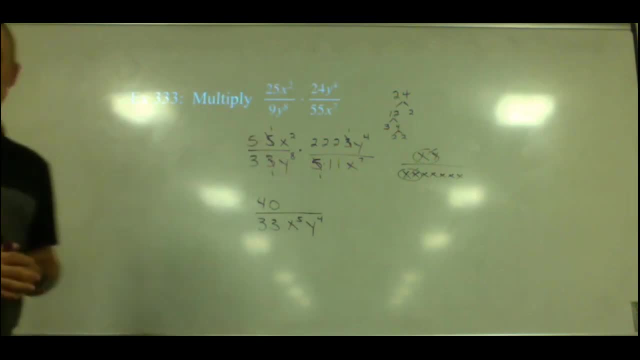 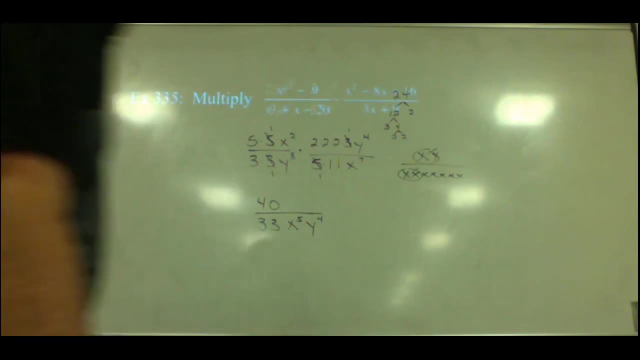 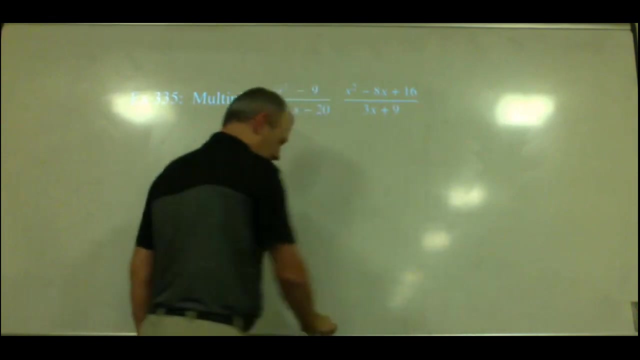 It's been a little while ago, But now we're going to be moving on to the new stuff, Which requires us to do a little bit more factoring, like we did in chapter six, So just like we were doing on those previous two examples. 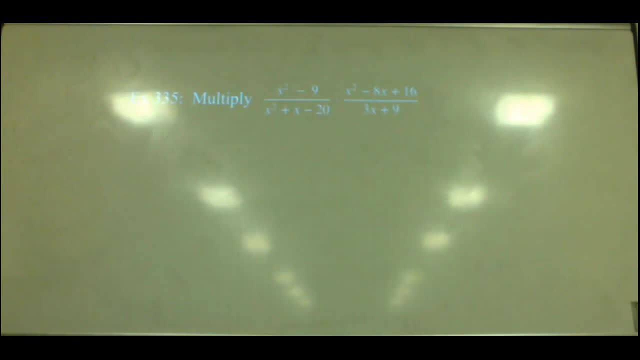 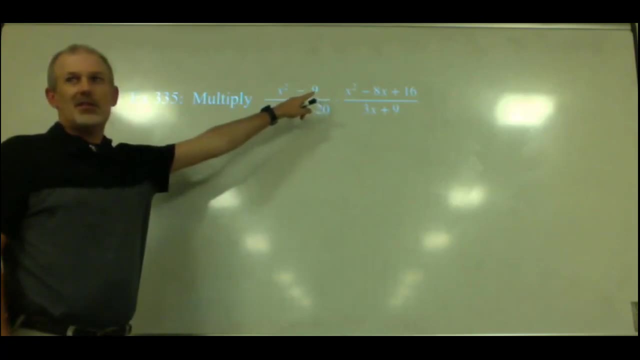 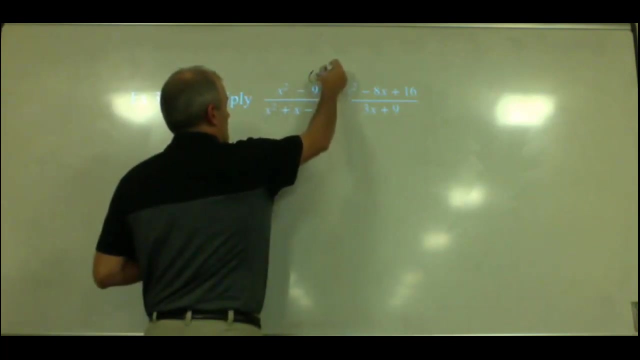 our first step is going to be always go ahead and factor: Okay, So x squared minus nine. That is one of our special patterns, And the reason it's a special pattern is because nine is, you know, three squared, And so that's the difference of squares. 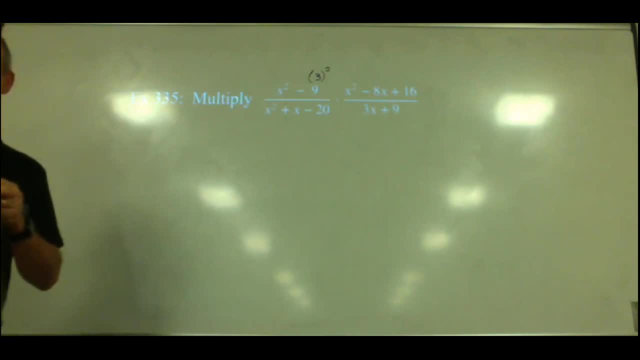 Okay, that's the one special pattern I said you probably want to learn this one. Do you remember how to factor x squared minus nine? Anybody remember that? You do like the x minus nine and then x plus nine. You're close. 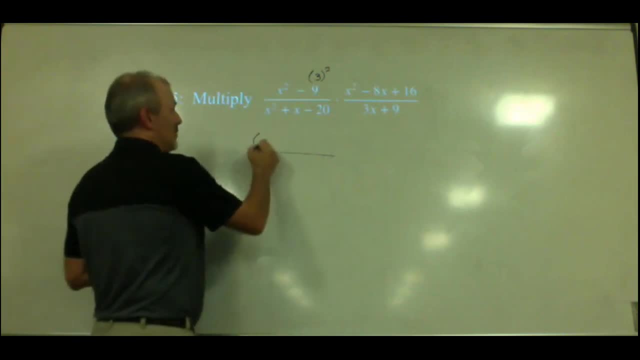 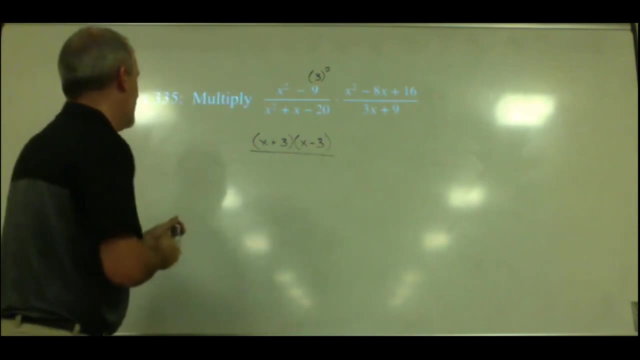 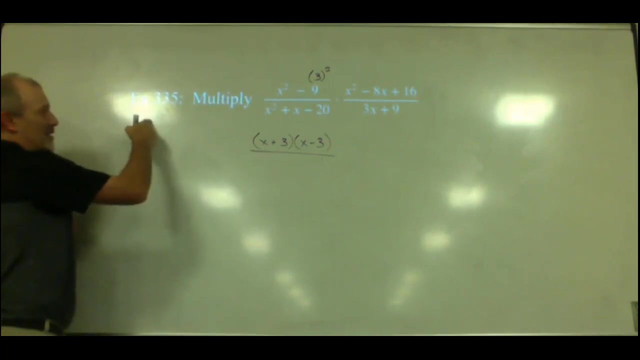 It's threes X because it's three squared. So it'll be x plus three and x minus three. So the pattern, if we want to remember the pattern, the pattern is: if you ever have a squared minus b squared, any perfect squares that are subtracted like this: 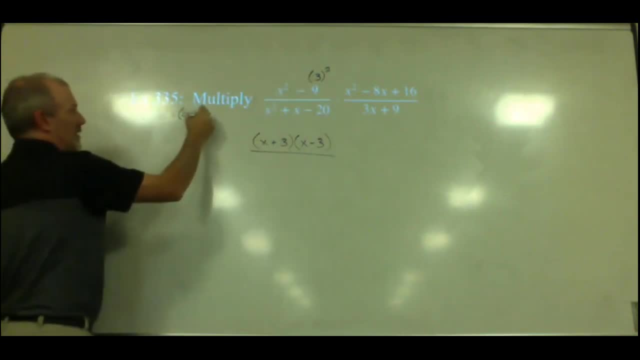 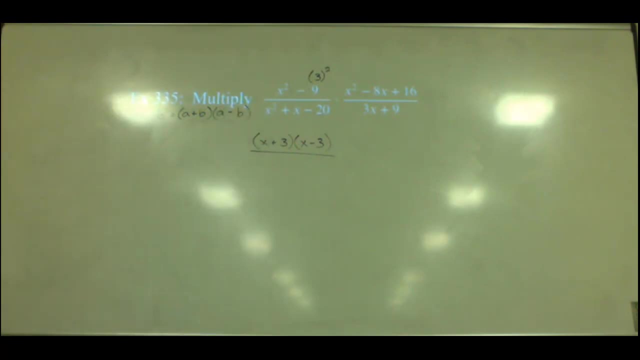 x squared minus three squared, it's always a plus b and a minus b. Okay, and that is one again that you probably want to remind yourself of, and go back to chapter six- I believe it was- And just review that a little bit. 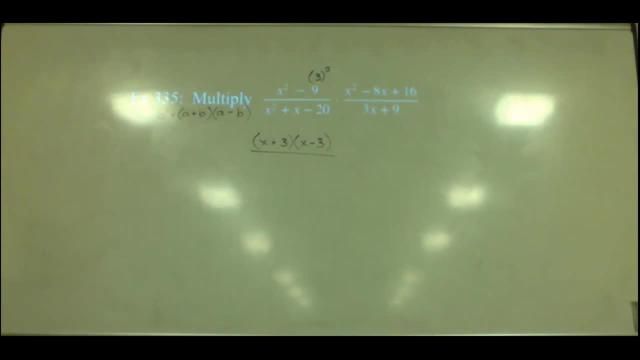 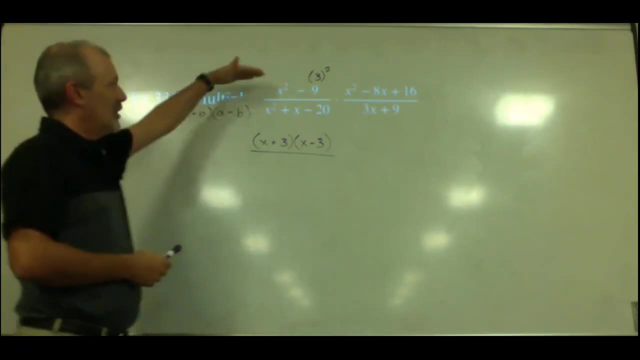 If you you don't want to get rusty in your factoring. That's why we did chapter six before. chapter seven is because we just keep using it from now on. Okay, so that's the numerator, Let's do the denominator here. 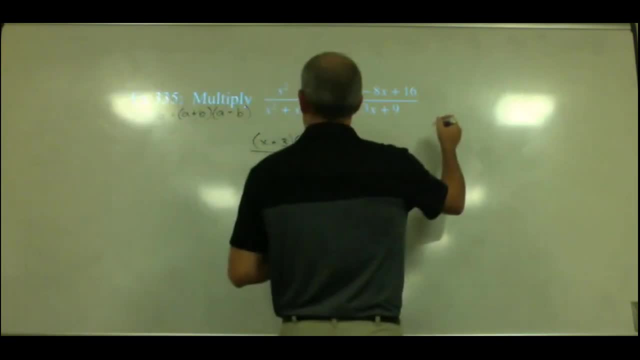 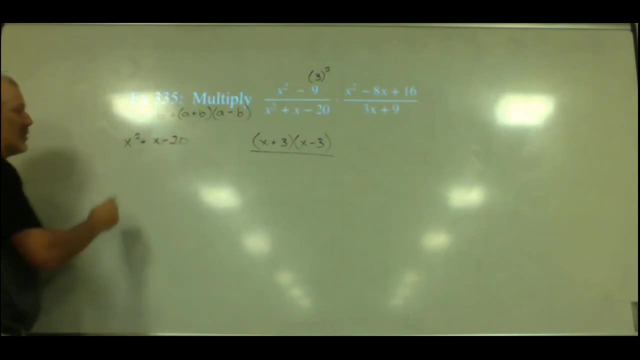 And we'll just go off to the side here and factor this one. So here let's go to this side: X squared plus x minus 20.. So remember our process. We take this number here, which is a one times that. 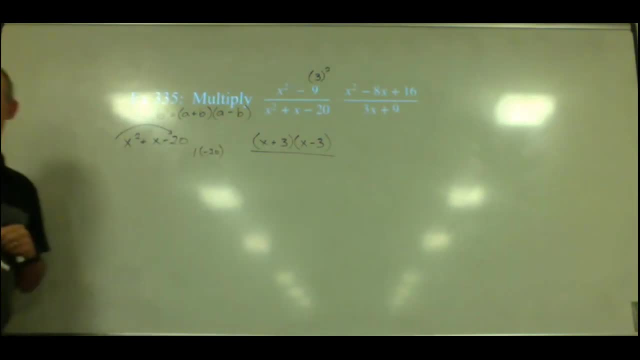 So one One times negative 20.. And one times negative 20 is Negative 20.. Negative 20.. I'm going to separate that, because here we're factoring Okay, negative 20.. Now we want to find factors of negative 20.. 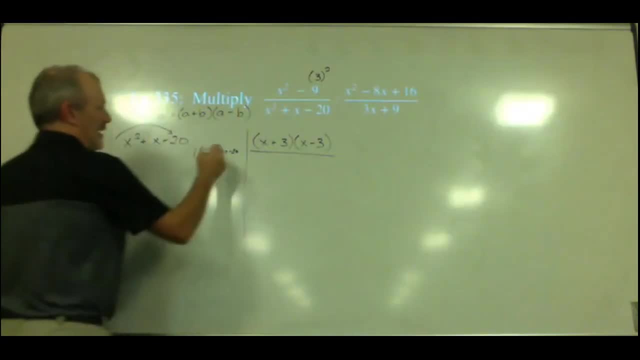 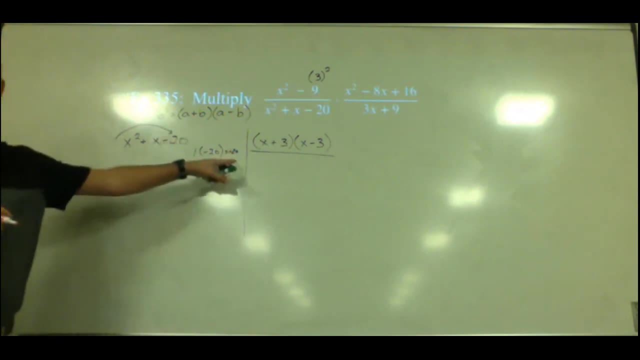 So two numbers that multiply together to be negative 20.. And since it is a negative, what does that tell us about the signs of the numbers we're looking for that are going to multiply together to be negative 20? Negative 20.. It tells us if you get a product of a negative. 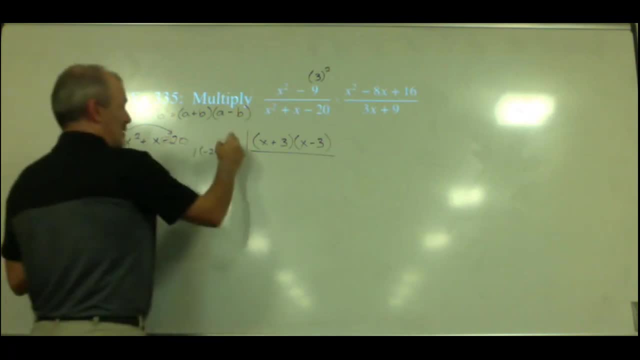 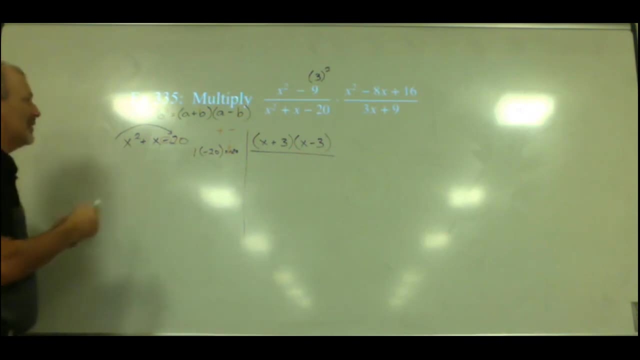 one has to be positive, one has to be negative. So that's what this tells us. This negative tells us one is positive and one is negative. Okay, Once we know that, then we can look at this one. And since they have to add together to be a positive number, 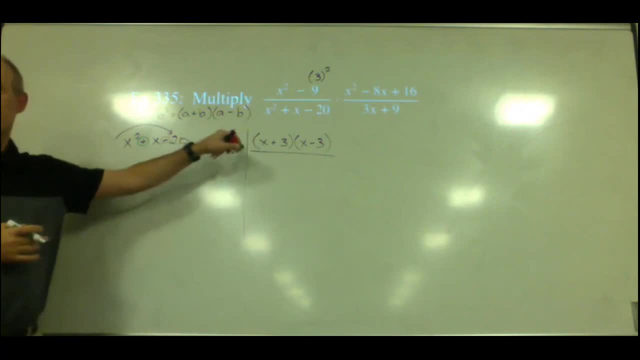 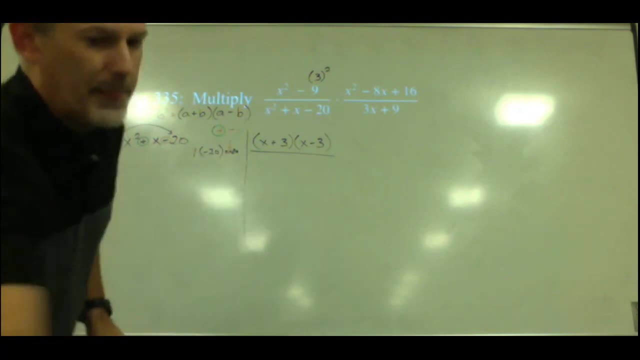 what does that mean about our positive and negative numbers? Positive is bigger than one. The positive one is the bigger one. Okay, so when we start writing out our factors of negative 20, we're going to make sure, when we write them out, the positive one is bigger. 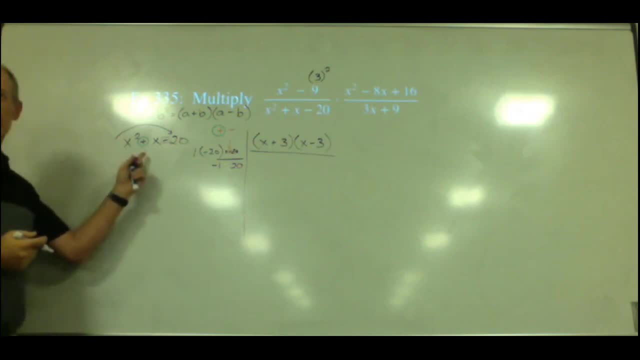 So we'll start with negative one with positive 20.. That doesn't add up to be one. Negative two times 10 is negative 20, but that also does not add up to be one. Three doesn't divide into 20,, but four does. 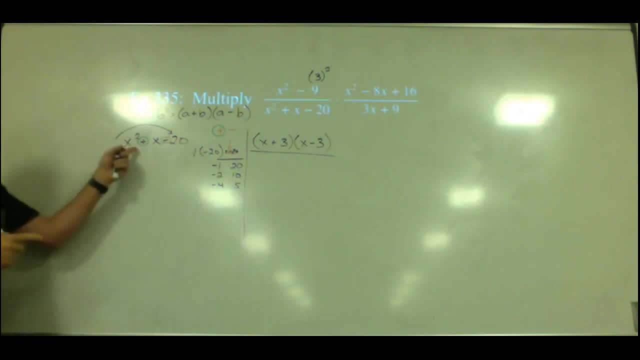 Negative four times five is negative 20, and that is positive one. So that's the one we need. Now remember what we do with those. We write this out as x squared minus four, x plus five, x minus 20.. And then get my red marker again. we factor by grouping. 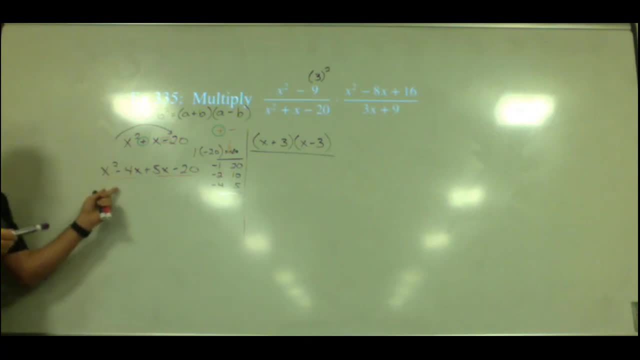 Okay, And if you look at this, what can we take out of the first group? What's in both of these? An x, right, They both have an x in them, So we factor out an x, And what do we have left? 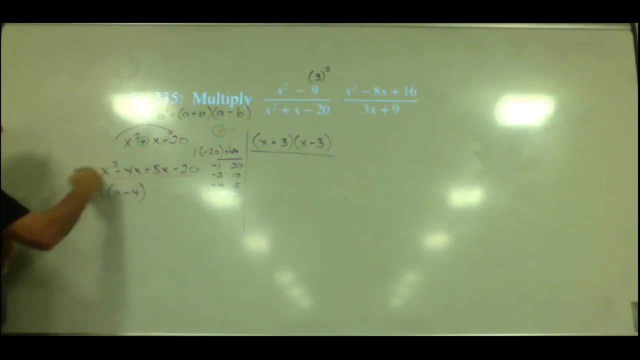 There's an x minus four. So we take out an x from each of those and you have x minus four. We have to take out this plus sign. And what else can we divide out of both of these Five? Five goes evenly into five and 20.. 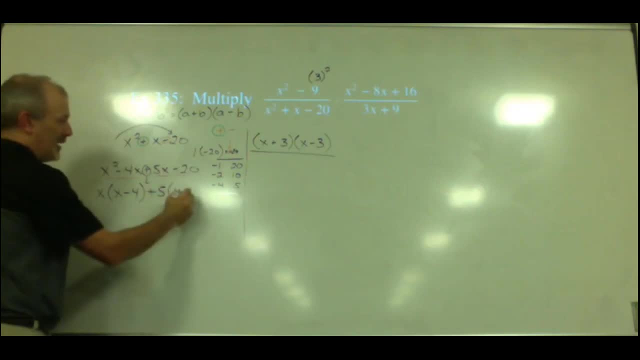 So what are we gonna have left? We'll have an x, and then 20 divided by five is four. So that means now that we have a factor of x minus four in each of those. we can take that out, and then we have x plus 5 left over. 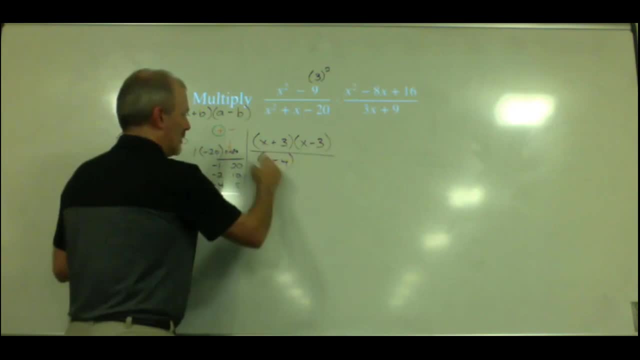 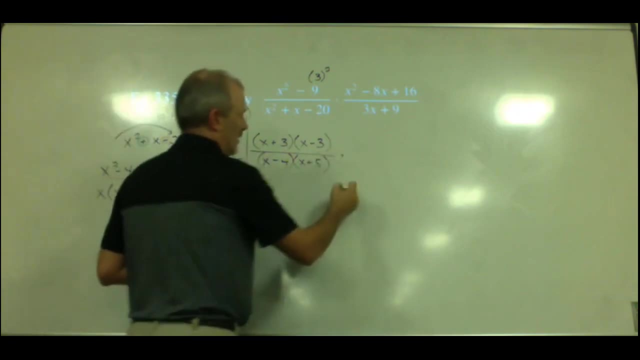 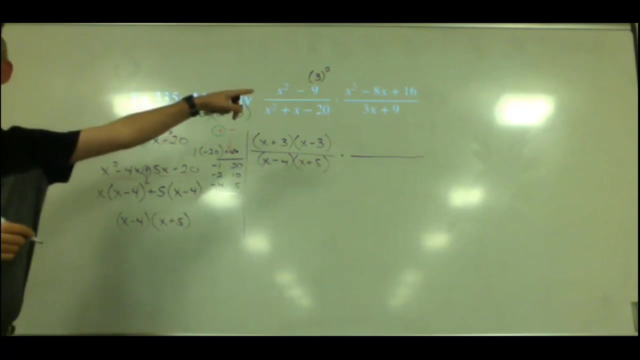 Okay, so x minus 4 times x plus 5.. So that's factoring that denominator there, times. Now we'll go to the second fraction and we're going to do the same thing on the top right. We need to factor that. 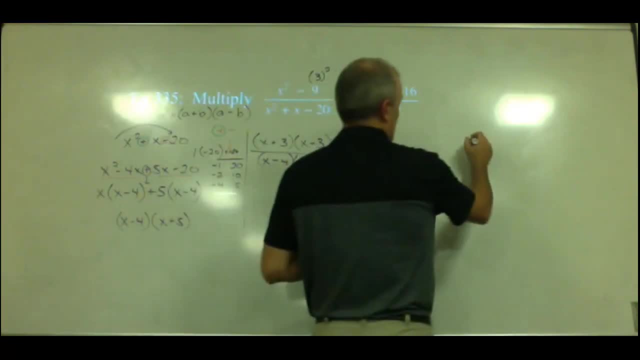 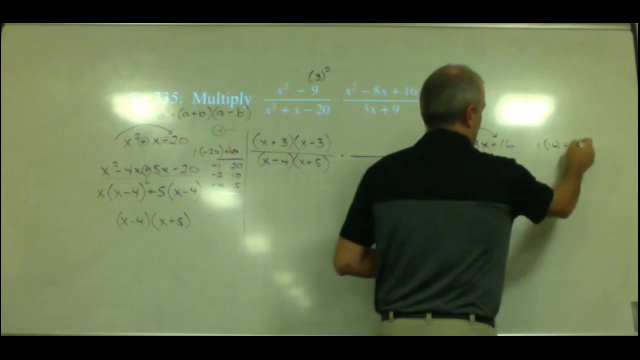 x squared minus 8x plus 16.. So let's do that over here. Make sure I'm still on the screen here. So we do the same thing: 1 times 16 is 16.. And this time, when we look at this, 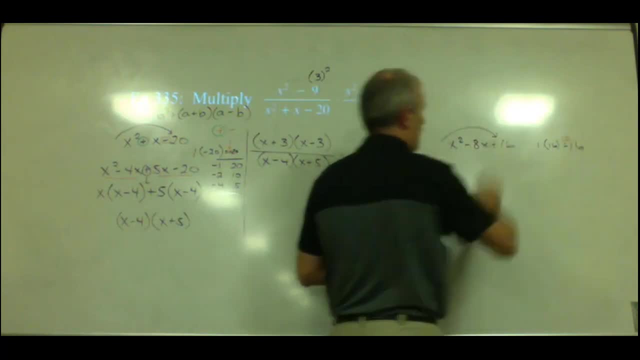 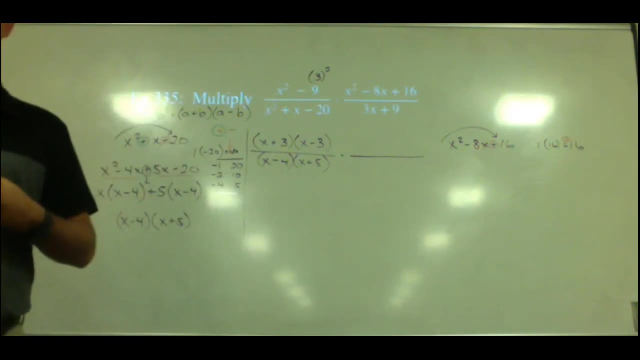 we see that this 16 is a positive 16.. And if we're looking for factors that multiply together to be a positive 16, what do we know about the signs? this time? There we go. They're either both positive or both negative. 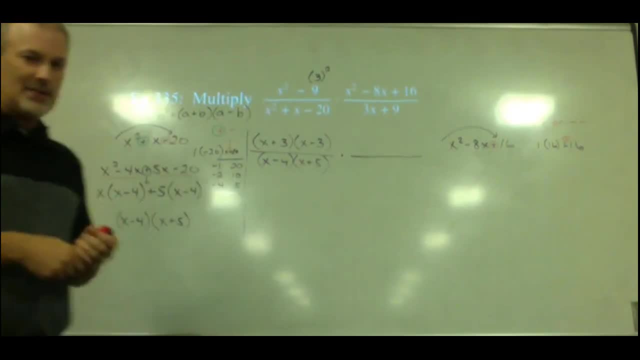 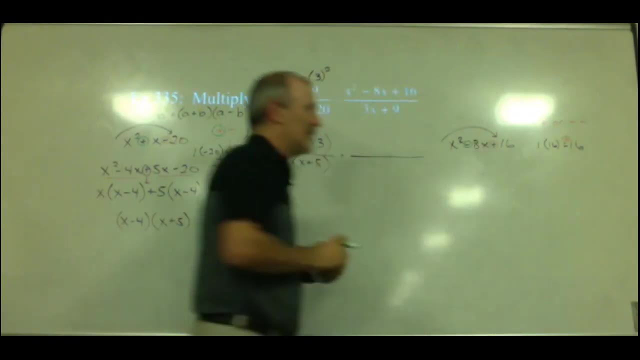 Okay, because if you multiply two numbers together and you get a positive answer- they're either both positive or both negative. Then when we look over here and we know that they add up to be a negative 8, that tells us they both have to be negative. 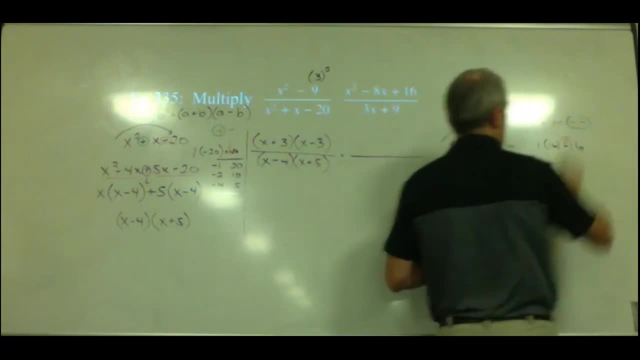 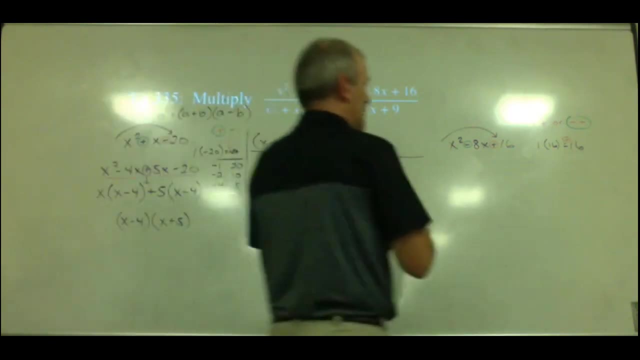 Because if you add two positives together you'll get a positive. Okay, So then let's go ahead and write out the possibilities. And they're both negative. So negative 1 and negative 16. multiply to be 16, but do not add up to be negative 8.. 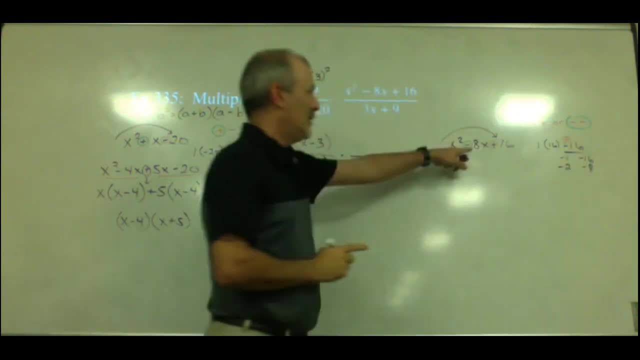 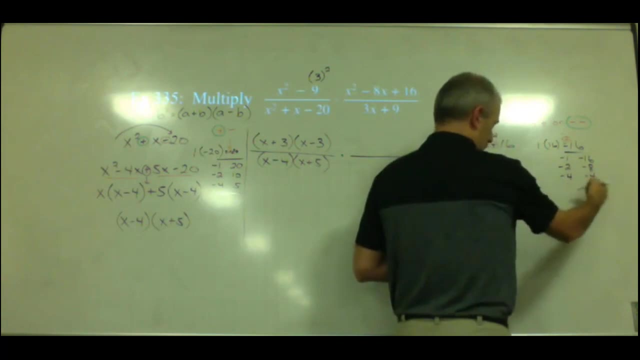 Negative 2 and negative 8 multiply to be 16, but they do not add up to be negative 8.. 3 does not divide into 16, but 4 does. So negative 4 times negative 4 is 16.. 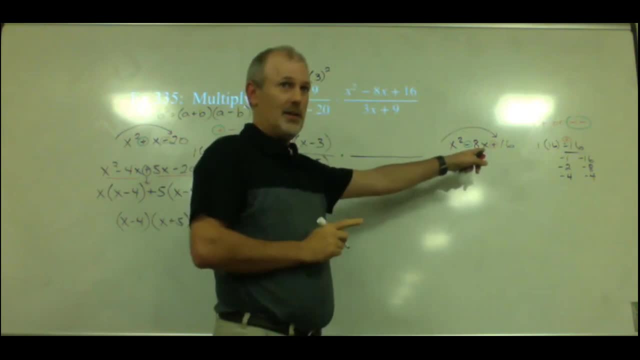 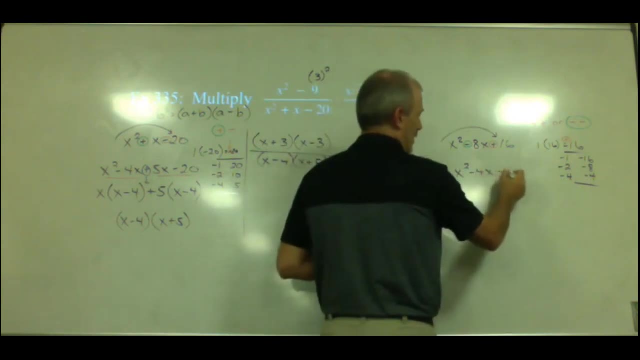 And negative 4 plus negative 4 is negative 8.. So those are, Those are the ones we're going to use, And we factor, We write them out and we factor by grouping again. So when we look at our first group, 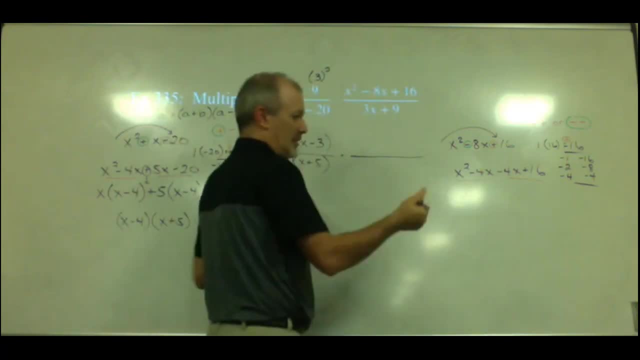 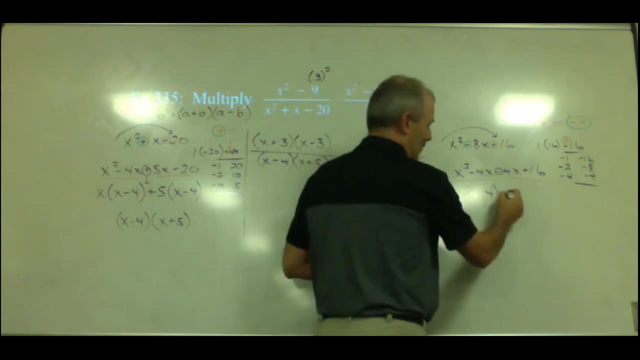 what can we take out of each of those X And X? And we have X minus 4 left. We have to take out the negative. And then, what else can we take out of the 4X and the 16?? A 4.. 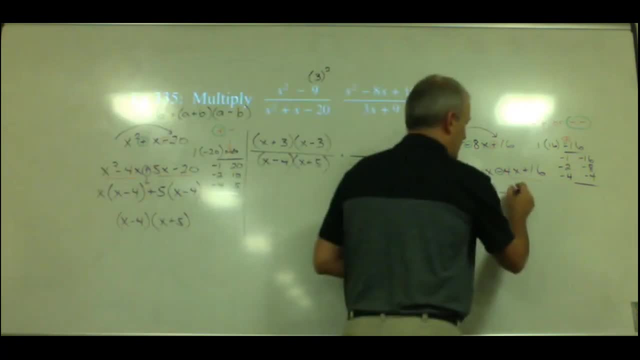 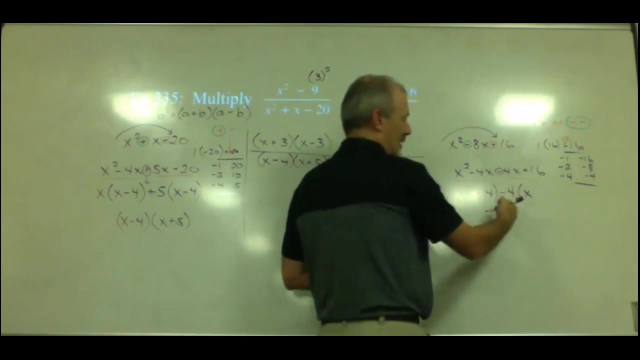 So we're actually dividing out a negative 4.. So negative 4X divided by negative 4 is just X, And then 16 divided by the negative 4 is negative 4.. So again, we need these to match up, And they should, if we did our work right. 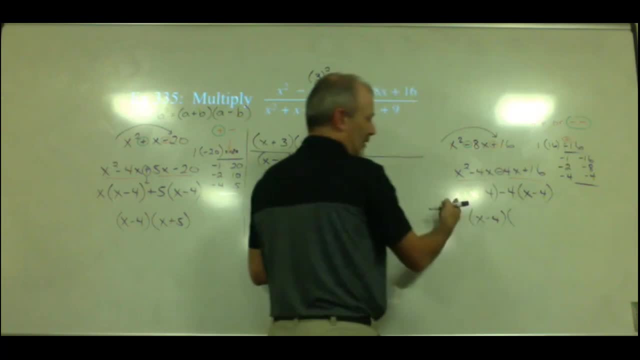 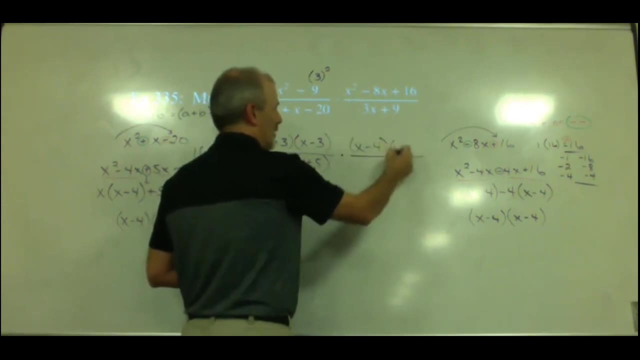 So X minus 4 can be factored out, And that will leave us with X minus 4 again. So those factors are both X minus 4.. So we have X minus 4.. And they should, if we did our work right, be X minus 4.. 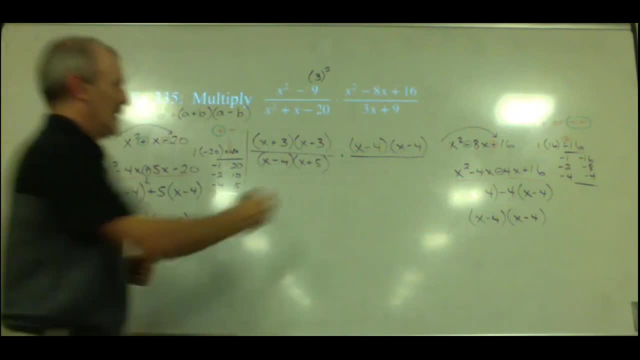 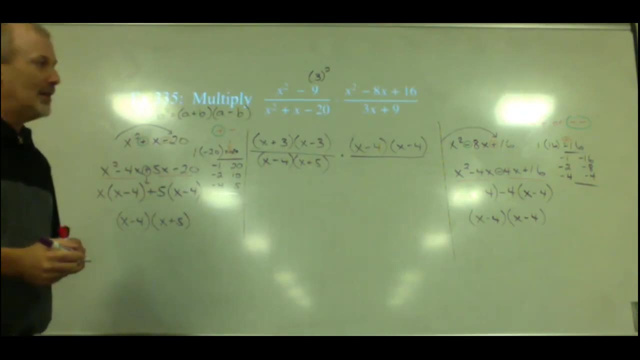 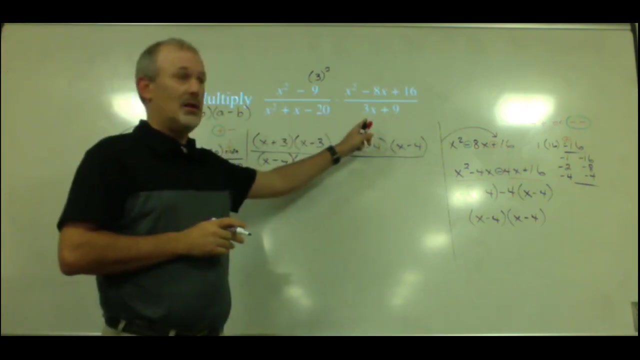 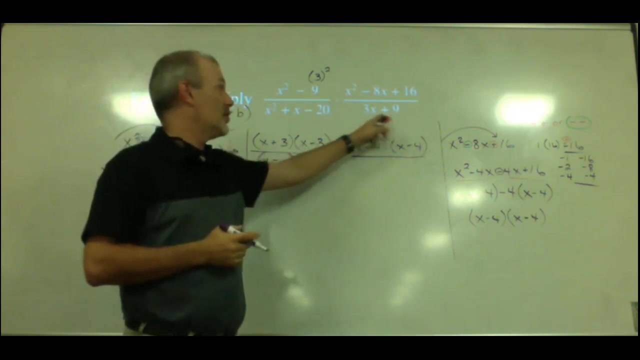 that's our factoring. okay, now the last one. don't be messed up by this. this is actually the easiest one because, notice, there's only two terms. we should always look for what first greatest common factor, common factor. so what can we factor out of both of these terms? 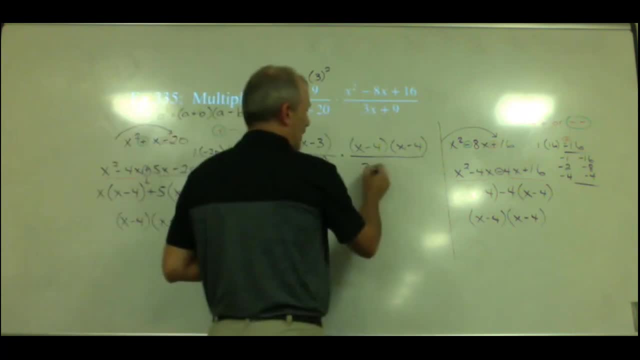 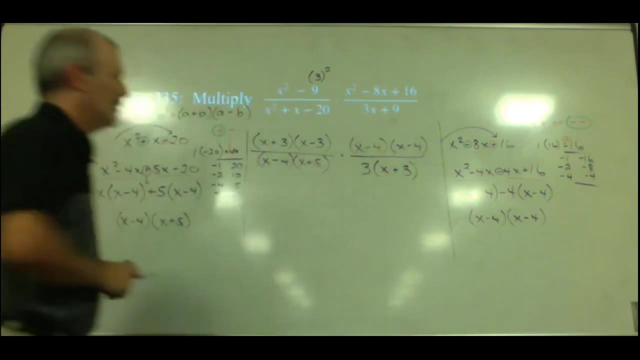 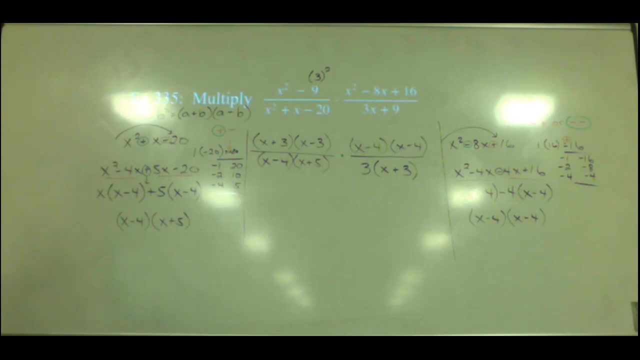 a 3. so we will factor out a 3 and then what's left inside there, X plus 3. okay, that's the hard part of this: factoring everything. once it is factored, then we look for our common factors. is there anything top and bottom that you guys see that we will be able to factor or we'll be? 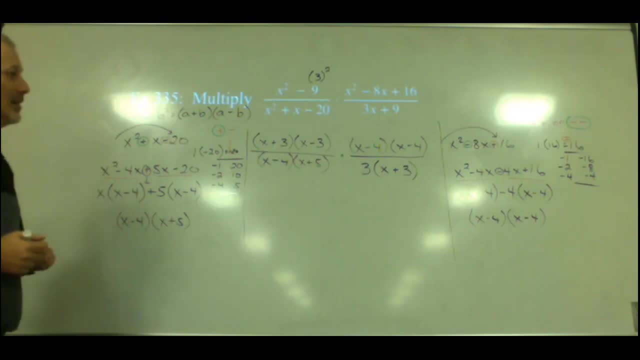 able to cancel X plus 3. okay, X plus 3 right here and cancel with X plus 3 down here. that's correct. anything else: X minus 4. X minus 4. do we see that? so X minus 4 down here can cancel with X minus 4 up there. 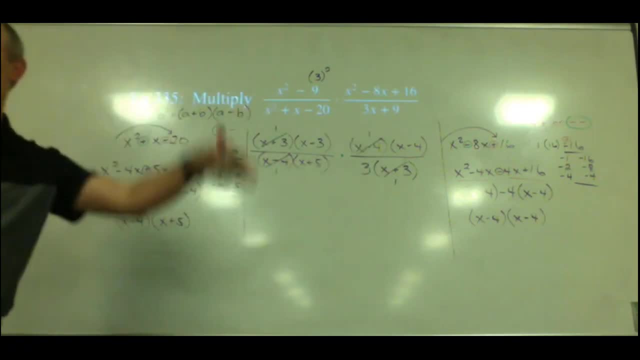 and it's got to be one with one. I can't cancel the X minus 4 with both of the X minus 4s. has to be one and one, one of each, okay, and it looks like that's probably everything now. when you write your answers, please do not multiply these all. 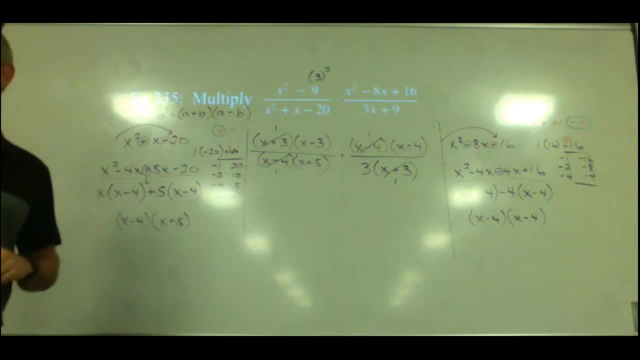 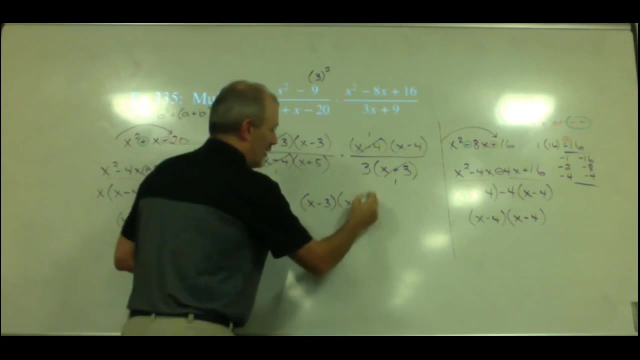 back out. okay, leave them. in fact, with numbers we multiply them back out, but with these, just leave it written as your answer would be X minus 3 times X minus 4 in the numerator, and then on the bottom you'd have 3 times X plus 5.. and that would be your answer. go ahead and leave it factored, don't. 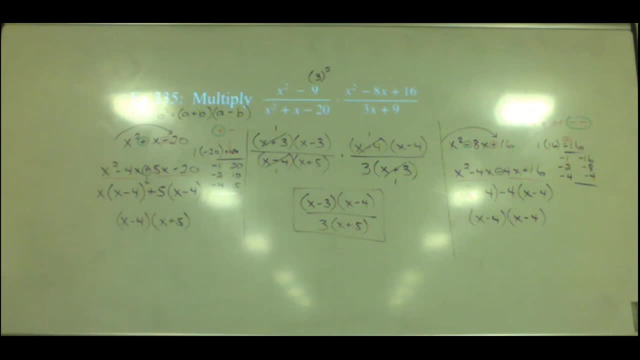 multiply it back out again. if you really really wanted to, you could, but that would use a lot of extra time that we are spending enough time just factoring, so we don't want to have to multiply it back out. and really, when you're doing problems like this, the goal is to eventually get to equations and 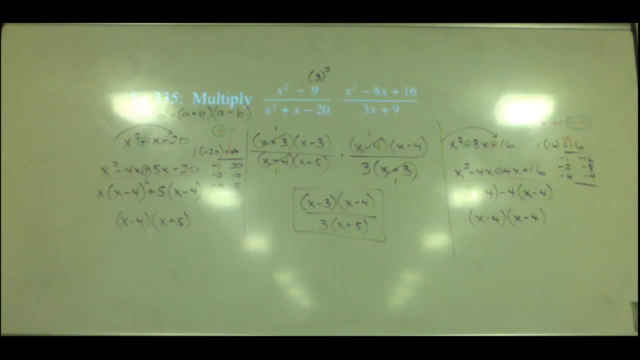 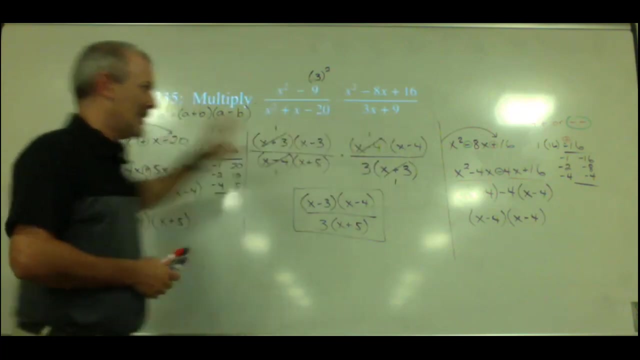 in equations. you're going to want everything factored anyway. we're not going to be doing any equations this year, this semester. okay, but does that process make sense? how we factor each numerator and denominator and once we've got it all factored- that's really the hard part- is the factoring once we've got it. 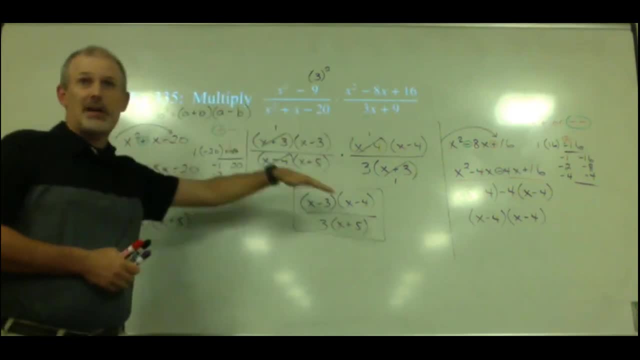 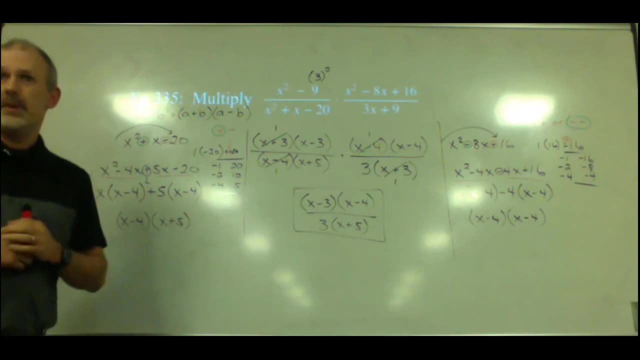 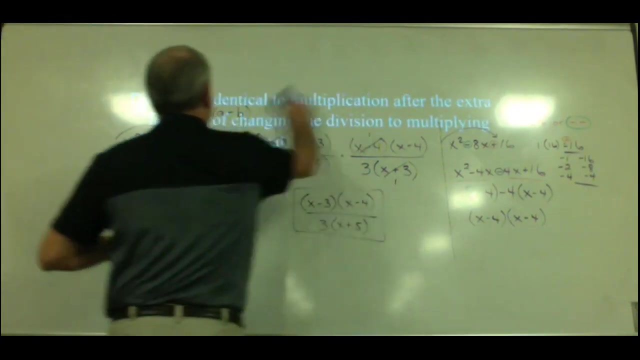 all factored, then we just look for what they have in common and we can cancel anything top to bottom. that matches up exactly. it has to match up exactly, okay. any questions before we go on? she's ready to go to bed. she's got her blanket, all right. so you had a rough day at work today. yeah, 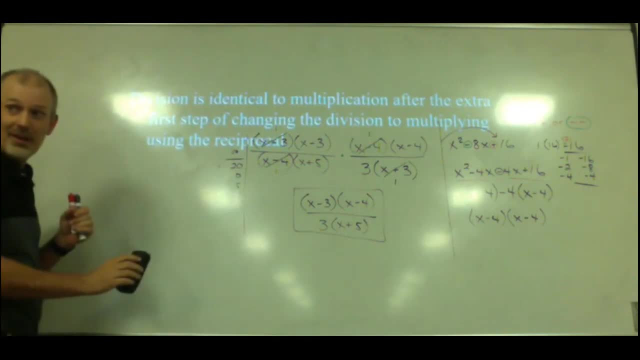 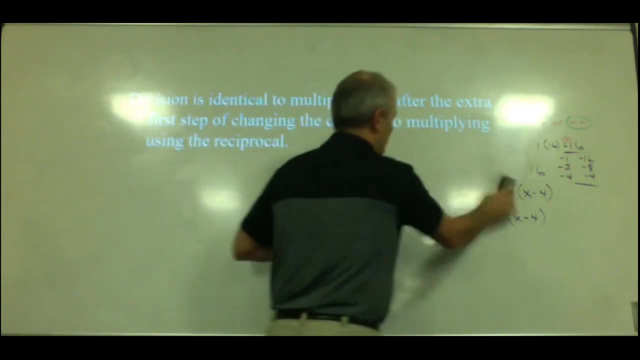 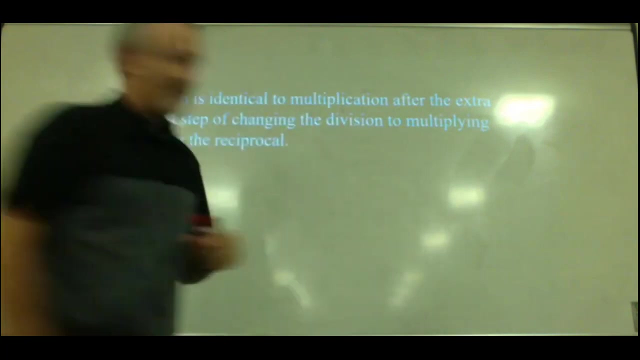 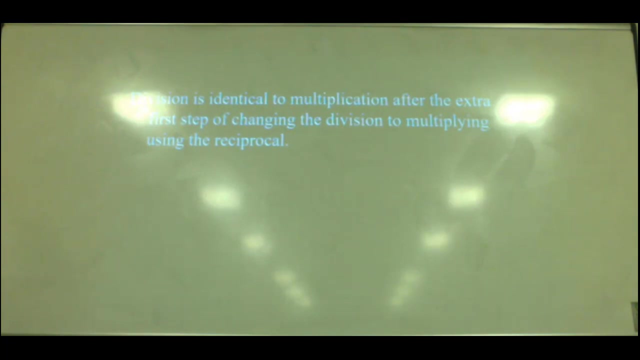 olog else to work always creates problems, and you did, you think you working human resources, yeah, and so that's probably even worse for you because that's, yeah, multiplication, but there's this one extra step that we have. The one extra step is- and again going back to 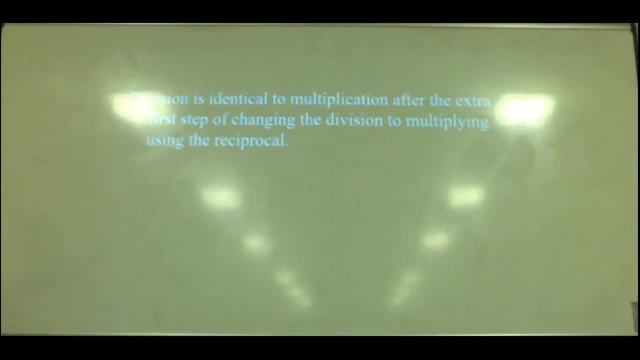 chapter zero. I don't know if you remember this, but with division of fractions. instead of dividing, we multiply by the reciprocal. And the reciprocal is where we take a fraction and we flip it and the numerator goes down to the denominator and the denominator goes up to the numerator. 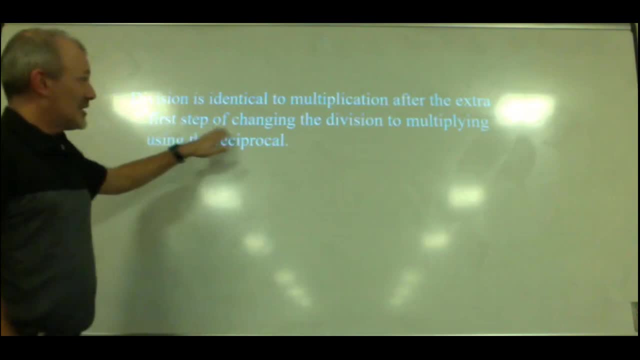 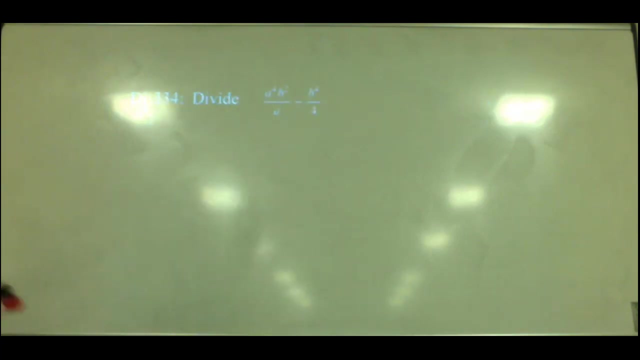 Okay. so when we do these, we're going to have this extra step of changing the division into multiplication by using the reciprocal. Okay, and you always do that. We do that with regular numbers and we do it with these rational expressions as well. So let's take a look. 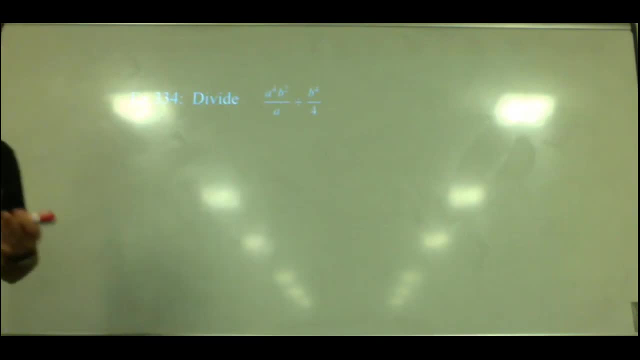 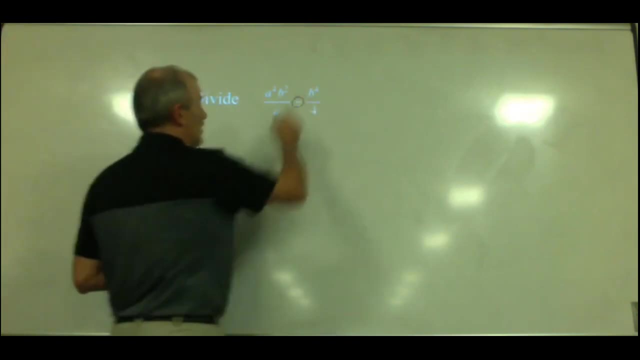 Again, just to remind ourselves of what's going to happen here, with a little bit easier problem. So let's do this The first step. anytime we see division, make sure you look for it. Anytime you see division, you're just going to copy down the first term, A to the fourth, B squared over. 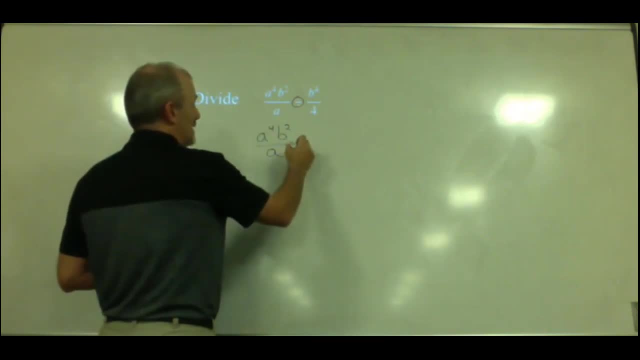 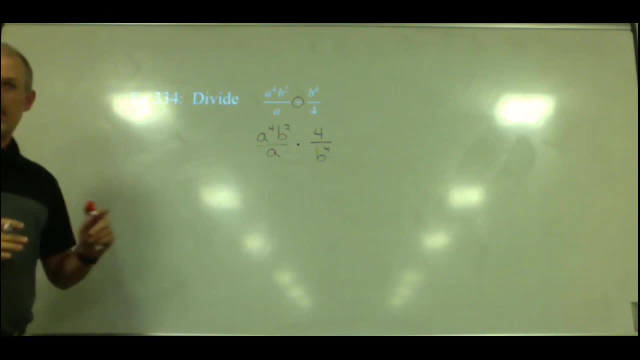 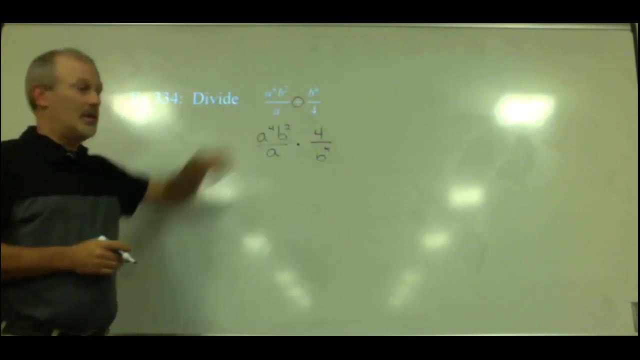 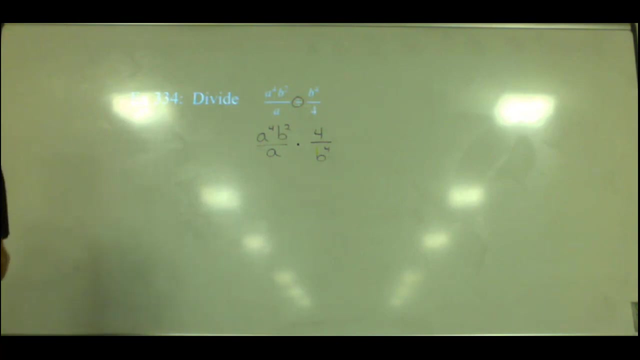 fourth. So does everybody see what we did with that second fraction? The four goes up to the numerator, the B to the fourth goes down to the denominator. Do you want to speak fast? Anytime you're dividing, that's the rule. so that we don't. we don't really have a good way of. 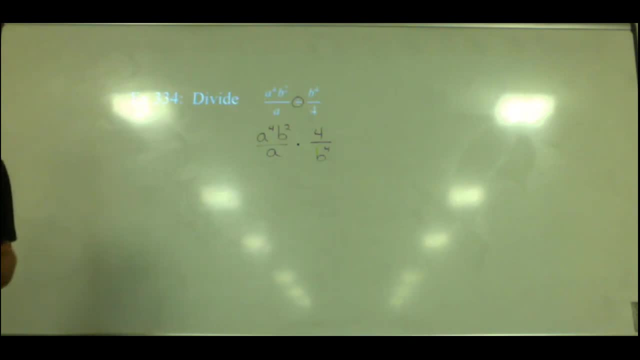 dividing fractions unless they're like perfectly matched up, like with specific numbers and stuff. So this is the same thing. It helps us. It just allows us to turn it into multiplication, Kind of like with subtracting. with sign numbers. we don't subtract, we switch. 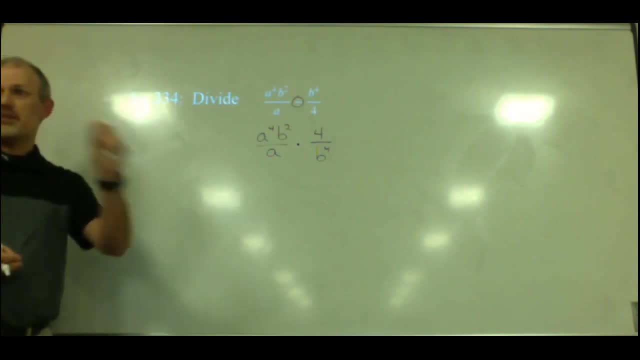 it into adding the opposite, because addition has a lot of nice properties and multiplication same thing. It has a lot of nice properties that division and subtraction do not have. So once we see it like this, what can we cancel? What do we see that we can cancel? 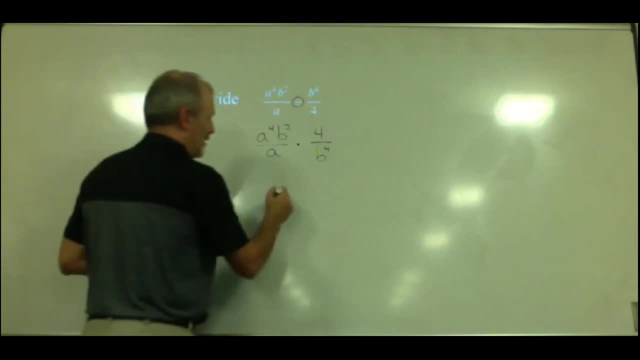 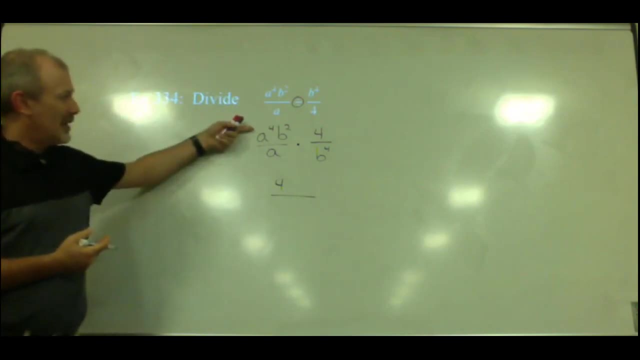 Notice we've got A to the fourth. Well, let's start with the fourth. So we've got A to the number. Notice the number. you've just got a four and it's on the top right. We just leave that there. We've got A to the fourth on the top. and this is A to what power? The first power, So what? 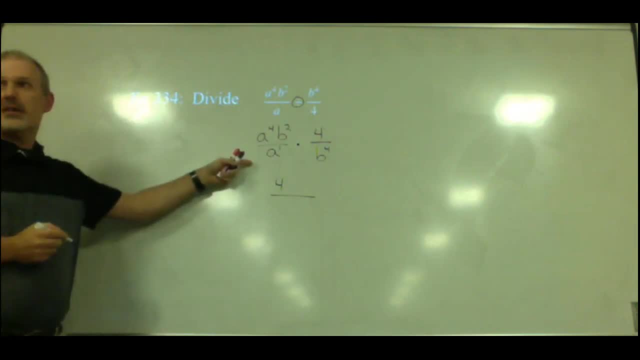 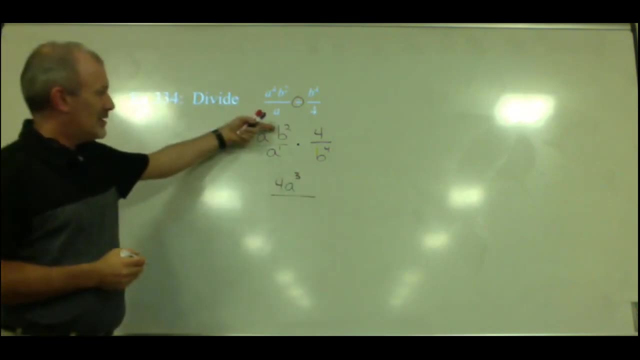 happens when we cancel those A's? A to the third power will still be on the top, So A cubed, And then we've got B to the second power and B to the fourth power. And what will we get when we reduce or cancel those? 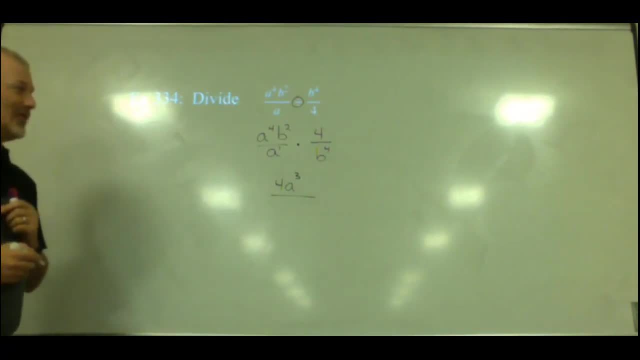 You subtract them, So you end up with how many left B squared? And where is it going to be In the numerator or denominator? It's on the bottom in the denominator. Okay, And that's as much as we can do. Once we've taken care of all the things that are in common, we're done, But this is the. 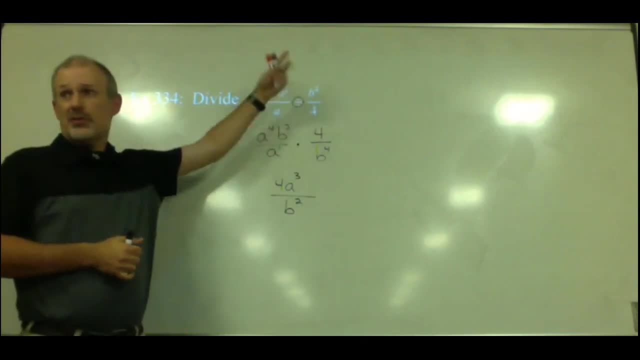 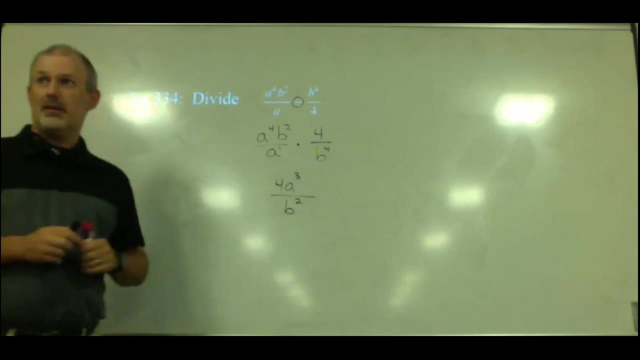 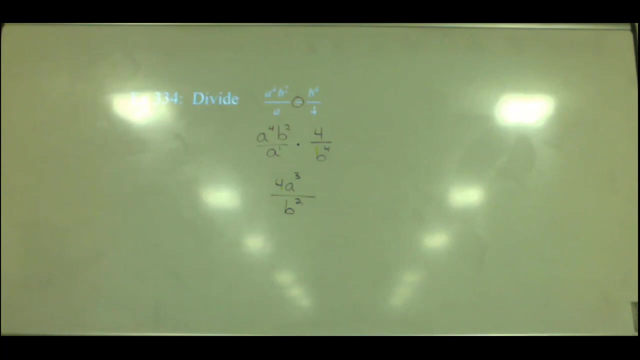 key thing, that first step. you have to switch it into multiplication And you do that by taking the reciprocal of whatever's. after that division: Yes, And that's the problem. We don't want to get that different answer, because that different answer would be wrong. Okay, So with multiplication we just do the work, But with division, 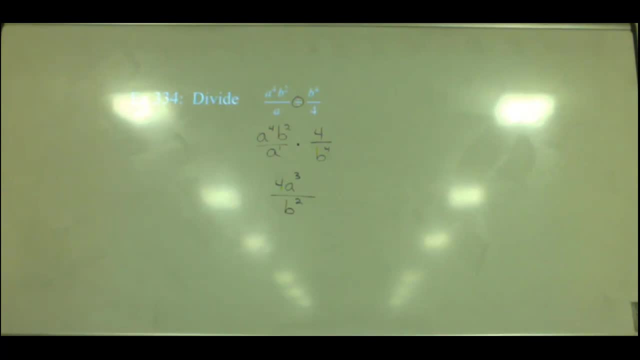 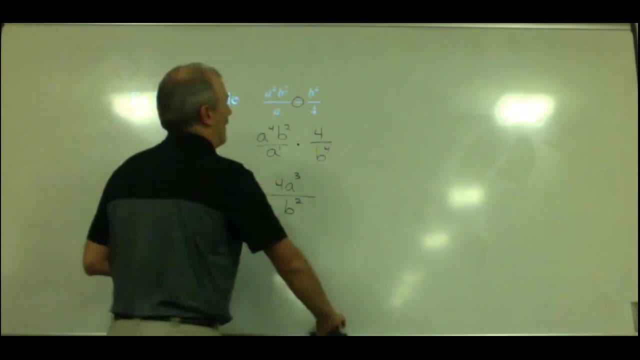 we have to take that reciprocal, and then we it's multiplication, and then we just do it. Okay, So we want to switch it into multiplication, because we already know how to do that. So that's it. That's it. I mean this one we didn't have to factor, So 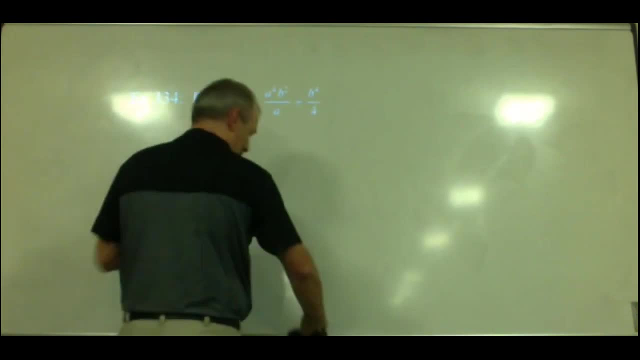 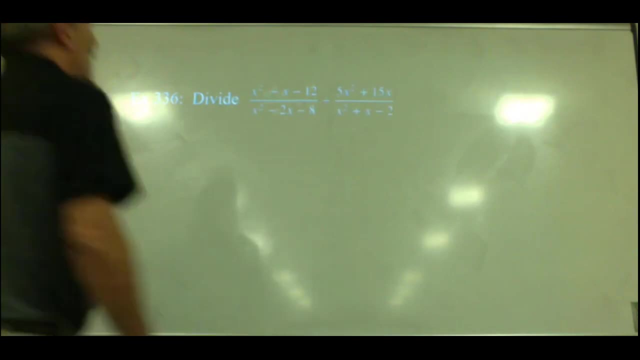 the ones that we're. this is like more of a chapter five question, but we're going to get to like these next ones where we have to actually factor something. Okay So factoring Here. we got more factoring, Okay, So let's start out. 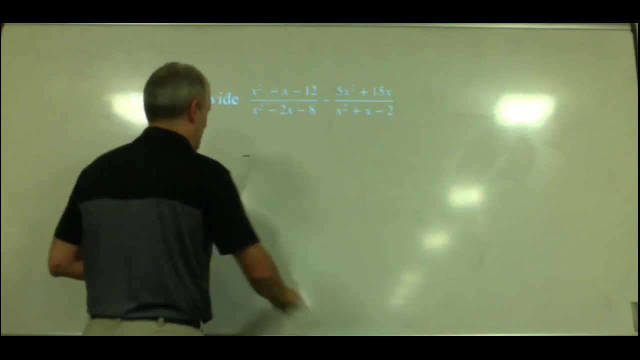 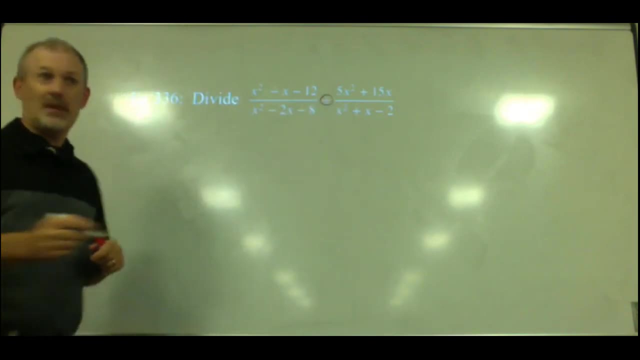 And the first thing, first thing I'm going to do- make sure I have space here- First thing I'm going to do is switch it into multiplication, right? So I'm just, I'm just going to copy down the first fraction: x squared minus x minus 12. 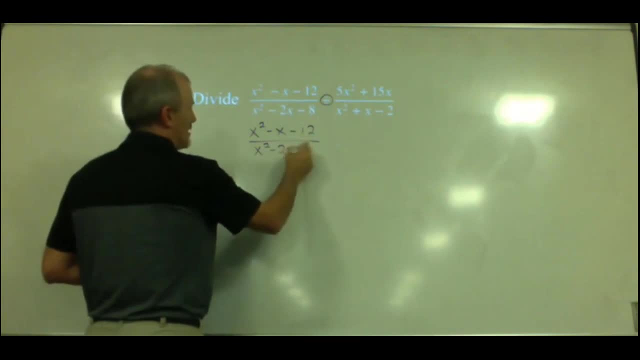 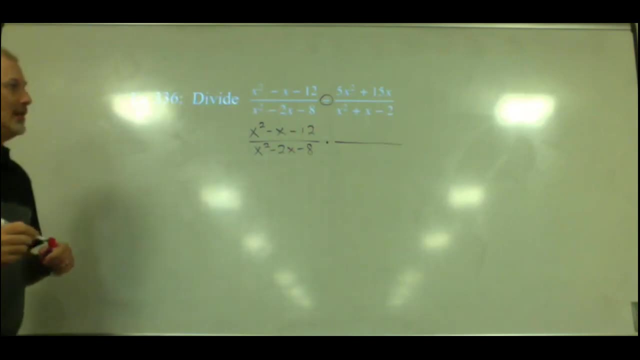 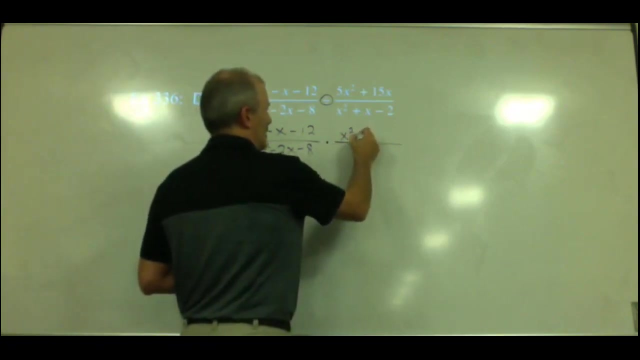 over x squared minus 2x minus 8 times. and then what will I put over here? What's going to go on the top, x squared plus x minus 2.. x squared plus x minus 2.. And on the bottom, that's going to be the 5x squared plus 15x. 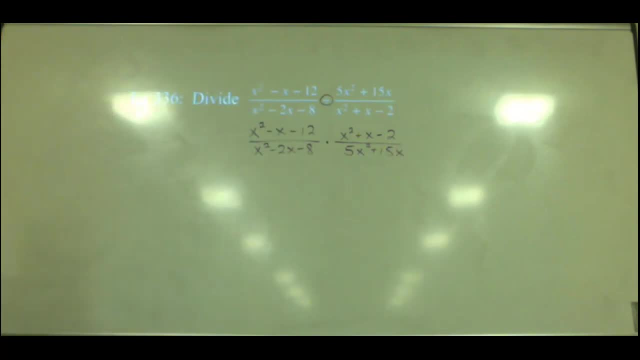 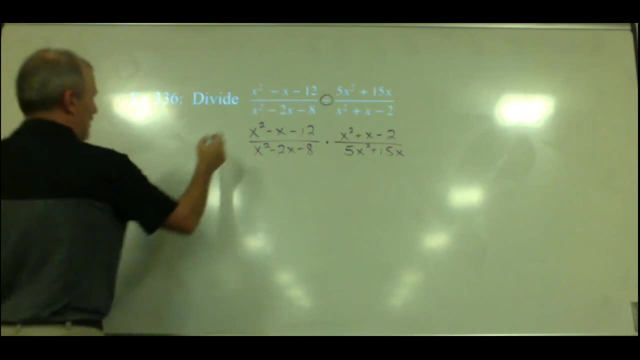 Okay, If you ever see division, that's your first step. Change it into multiplication. Okay, Then we have to do our factoring, and we've got lots of factoring here. All right, Let's start with this one on the top: x squared minus x minus 12.. Remember: 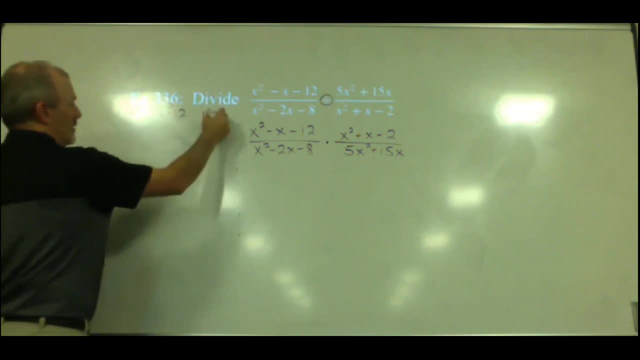 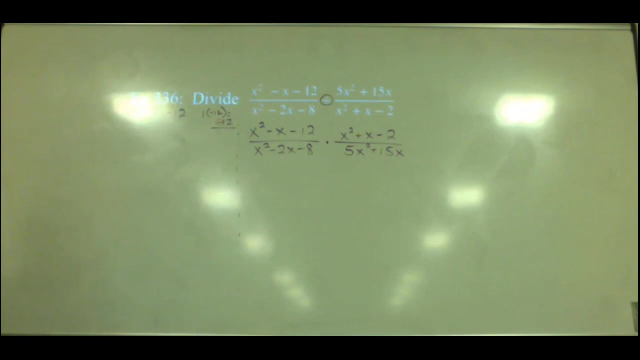 we multiply 1 times negative 12, and that gives us negative 12.. So we're trying to find factors of negative 12.. What does this sign tell us, since it's negative? What does it tell us about the numbers that we're looking for? 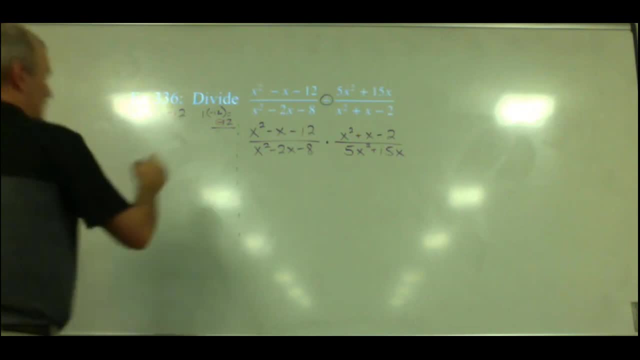 One negative and one positive. One is negative and one is positive, And so I'm going to put that right up here: One positive, one negative. Then, since we've already dealt with that sign, let's deal with this one. What does it mean to us that the negative sign is in the middle there? 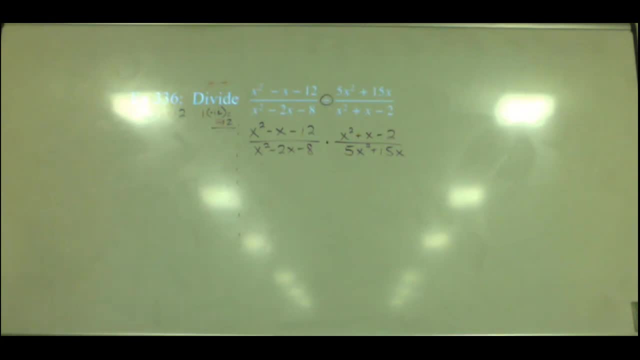 It needs to be negative, Negative, Negative, Negative, Negative. The biggest number needs to be the. The bigger one is negative, because when you add them together you get a negative answer Right. So the bigger one is going to be negative. So when we start writing out our factors here, 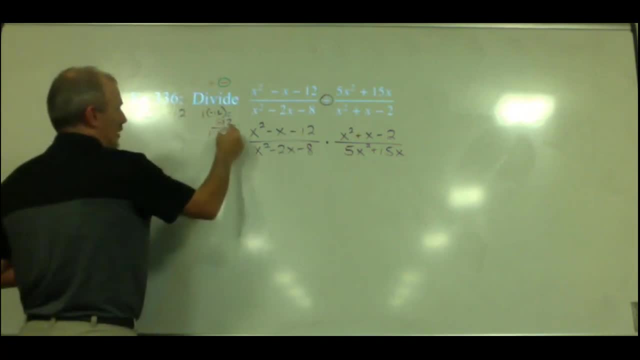 we're going to have the bigger one be negative, So positive one with negative 12.. Does that work? No, No, that doesn't add up to be negative one, Two and a negative six would be the next pair. Does that work? 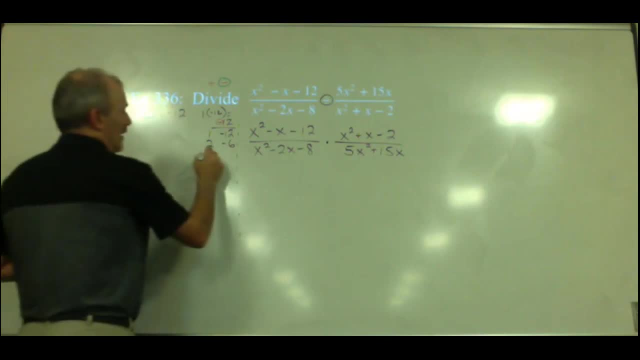 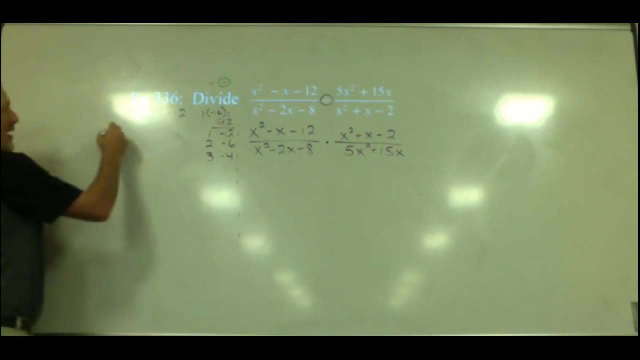 No, No, because that's negative four. Yeah, That's negative four. Three and negative four is the next pair. Does that work? Yeah, Yeah, So we're going to have x squared plus three, x minus four, x minus twelve. Okay. 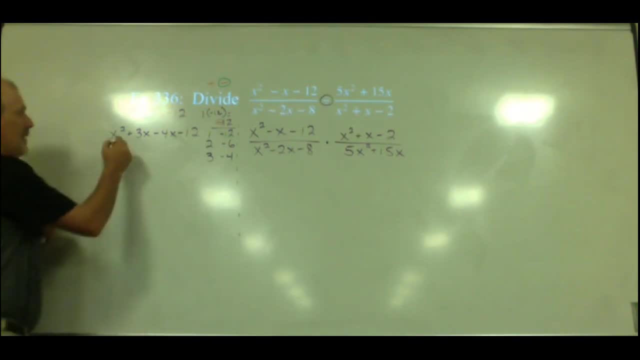 Then we are going to factor by grouping And I want to show you a little short cut tonight that maybe you guys have kind of already realized, or maybe you haven't. You guys can do that, haven't. But we're going to finish this first and then I'm going to show it to you. What can we? 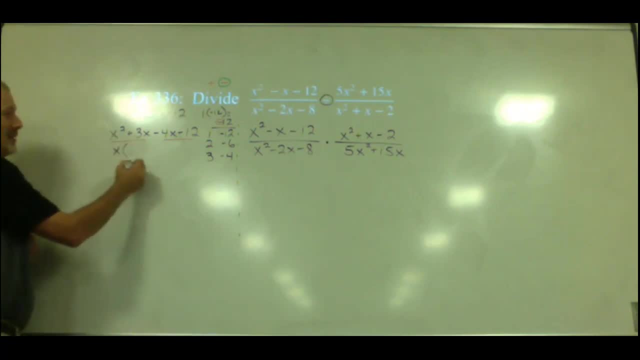 factor out of the first group, X, And what's left? Correct, X plus 3. Then we have to take out the negative. And what else can we factor out of that second group, A, 4.. Yeah, So we're dividing out a. 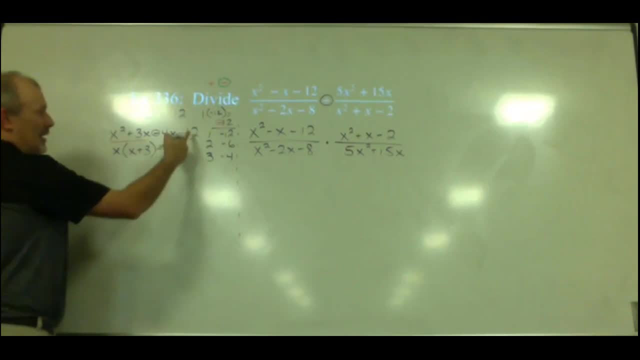 negative 4.. Negative 4x divided by negative 4 is just x. Negative 12 divided by negative 4 is plus 3.. So we can factor out the x plus 3.. And then what we have left is this x right here and the. 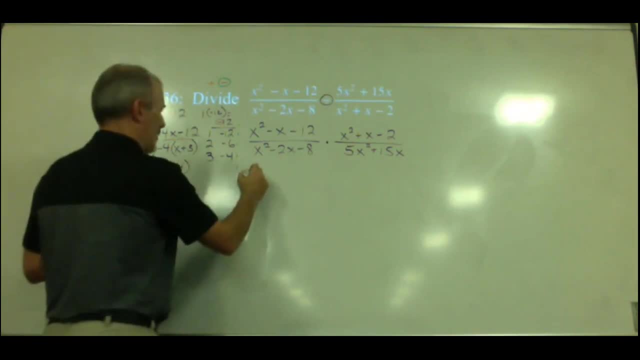 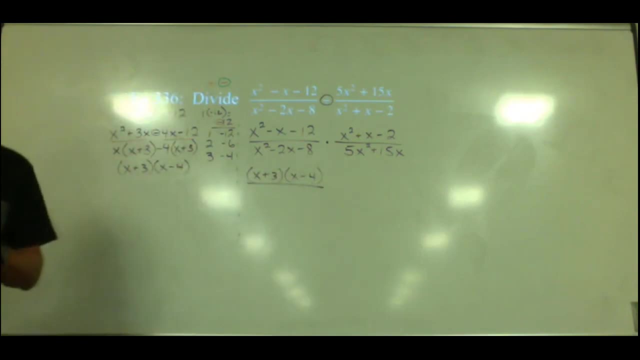 minus 4.. So that is going to be our numerator: X plus 3 times x minus 4.. Now what I want to show you as a shortcut, and again, you may have realized this already or you may not have, but anytime, this first term is just an x squared. 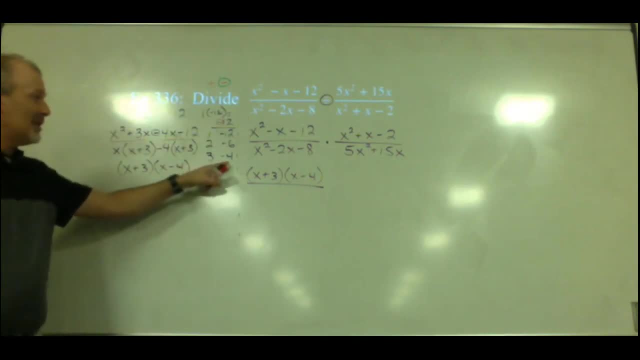 you're going to have to do the same thing, So you're going to have to do the same thing Once we get these two numbers here. notice how these two numbers compare to these two numbers When this is just an x squared. once we get these two numbers, we can actually just put: 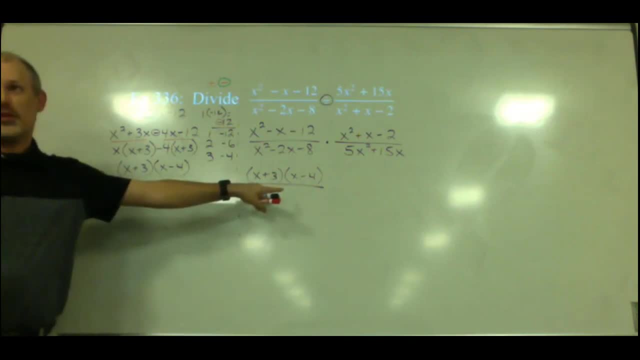 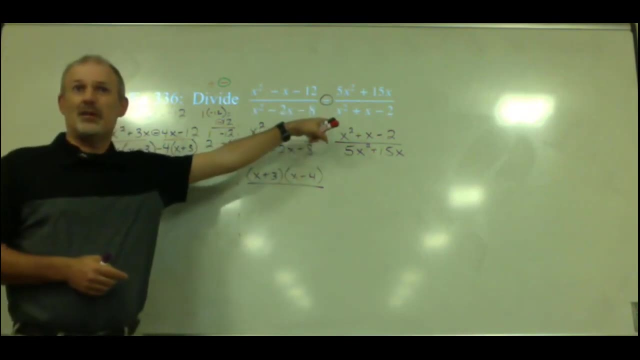 them in the parentheses and we're done. So it saves us. It's a shortcut. It only works if this is just an x squared, But notice, a lot of these are just x squared. So it's going to save us some time. But if you're not sure, then just do the factor by grouping. You'll still get the same. 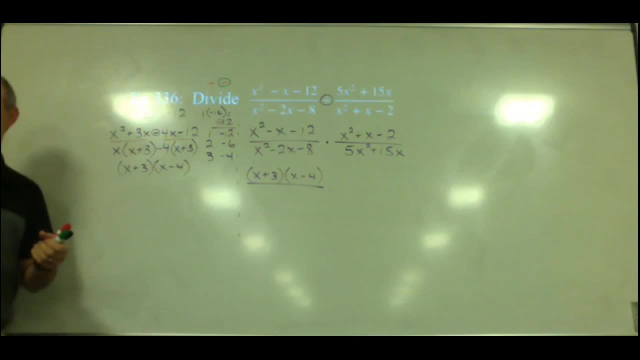 answer. It's just again. it's a shortcut that works as long as these are just x squared. So we're going to try and see if we can use that tonight. to save a little bit of time. Let's go ahead and do the. 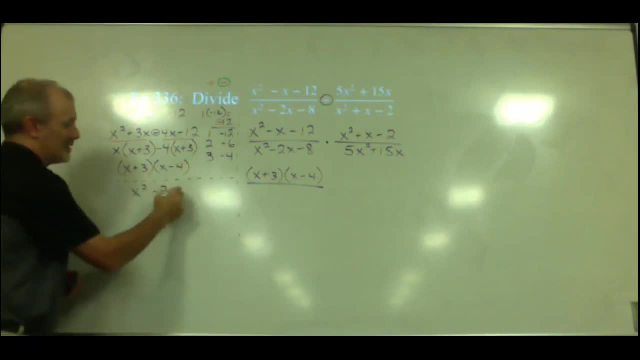 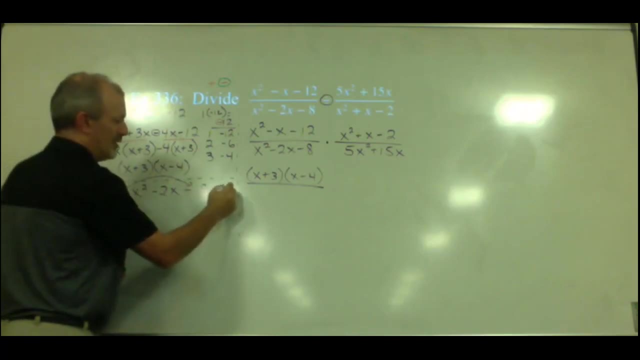 bottom x squared minus 2x minus 8.. So we're going to take the 1 times the negative 8, which is negative 8.. We're still going to do all of our examination. So, whether it's this one or 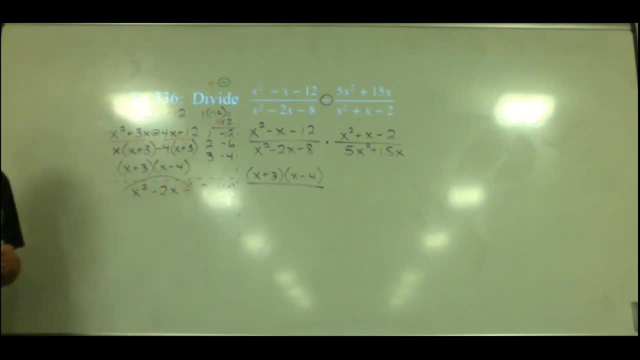 this one. we're going to do all of our examination. So, whether it's this one or this one, what does it mean that that sign is a negative, One positive, one negative? And then, once we look over here, what does it mean that this one's negative, Bigger one's negative? So this is. 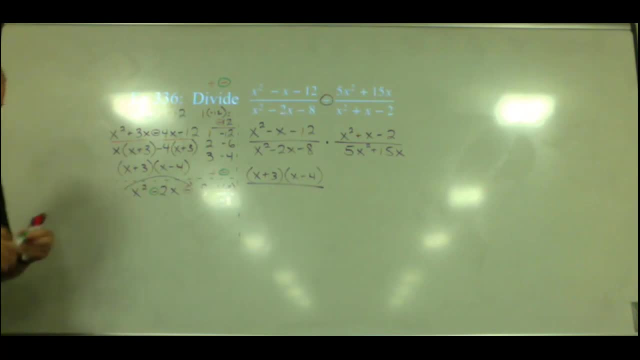 actually kind of the same setup we had in the previous one. So let's see if we can find the right pair. So the bigger one's negative 1 and negative 8, does that add up to be negative 2? Nope. 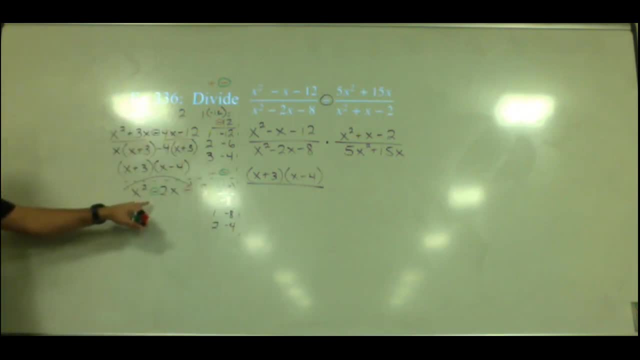 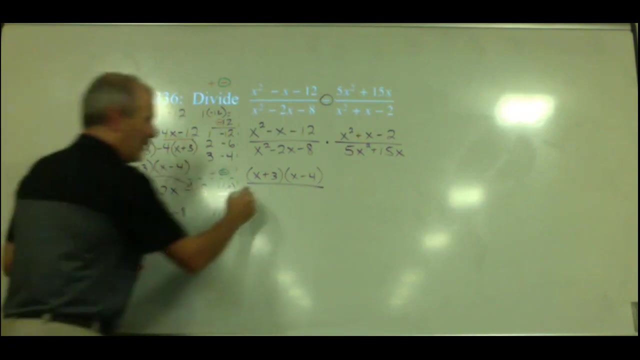 2 and negative 4, does that add up to be negative 2?? Yes, Yes. So here's where we're going to do our shortcut. Instead of writing it out as x squared plus 2x, minus 4x, minus 8,, we're going to jump straight to the fact that we know because we've 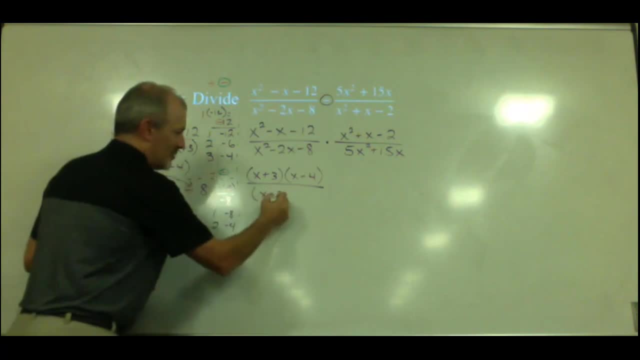 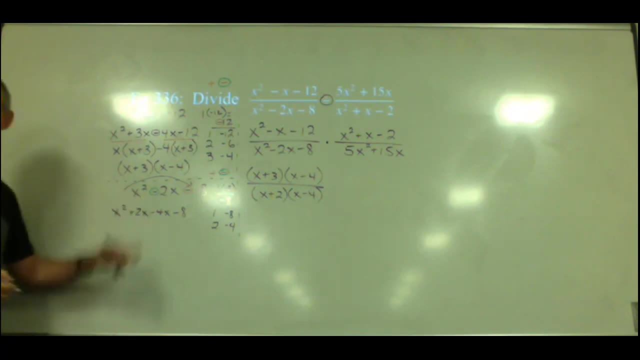 done a lot of these. we know that this is going to become x plus 2 and x minus 4.. So that saves us the fact that we have a negative 2.. So we're going to do our shortcut. So the second thing we do is we have our vector by grouping part, If you want to. 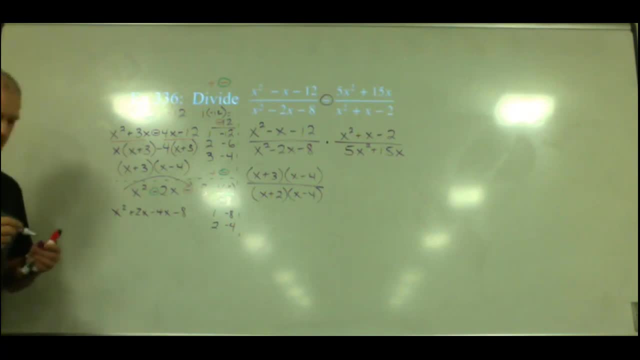 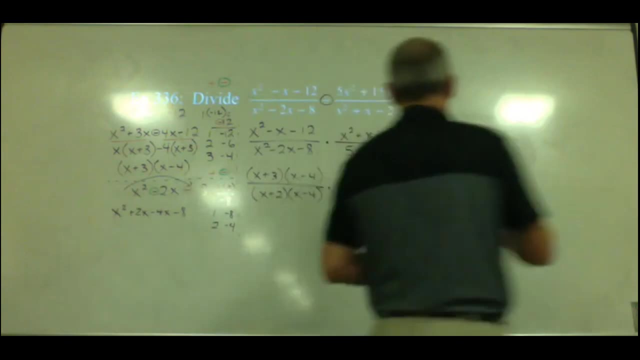 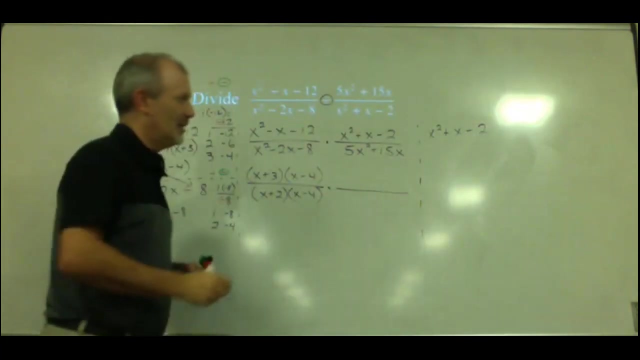 factor by grouping. go ahead, but this will save you a little bit of time. Now let's do the second set of fractions. We've got x plus squared, plus x minus 2.. This one will be a little bit easier, Because 1 times negative 2 is negative 2.. 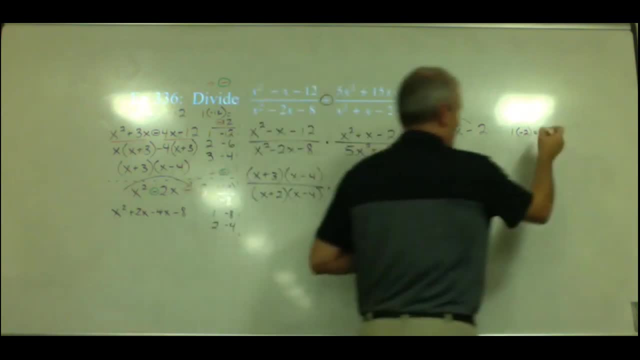 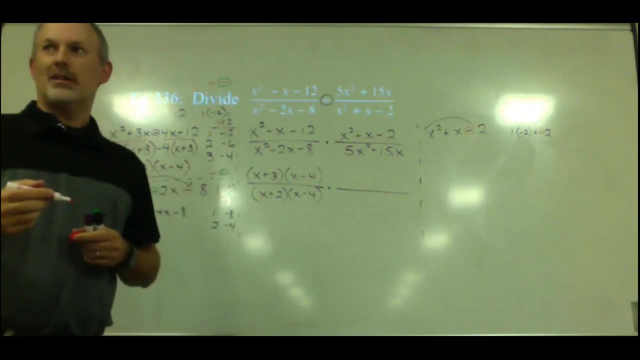 And and. What does this negative sign tell us? once again, How about the numbers that we're looking for? The signs are different. Notice, it's been actually on all three of these it's been the same thing. The signs are different. 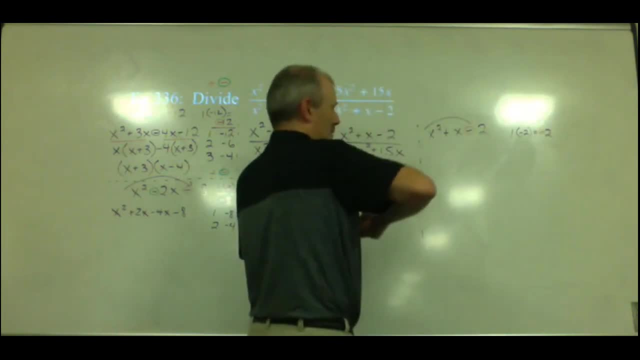 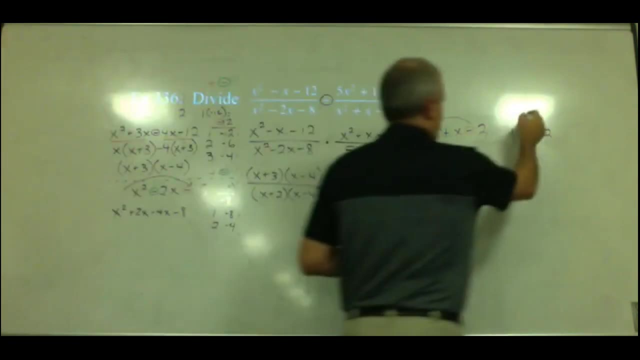 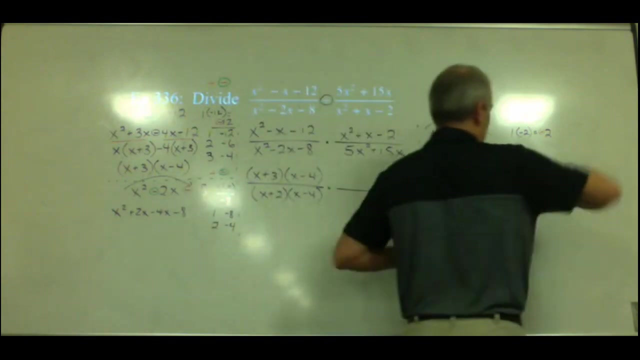 But this time this middle one is a positive. So what does that tell us? The bigger one is positive. Okay, so when we find our factors of negative two, this time the bigger one is positive and actually we only have one option. 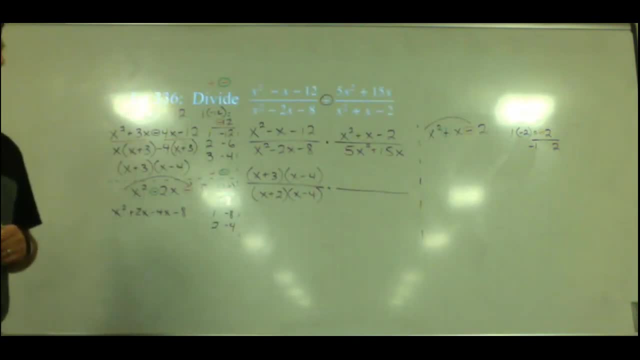 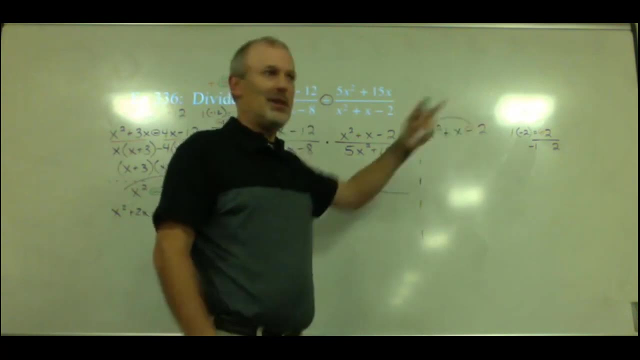 because two is prime And does negative. one plus two add up to be what we need. Yeah, it adds up to be one right, And that's what we needed. So again, we can use our shortcut, since this is just an x squared. 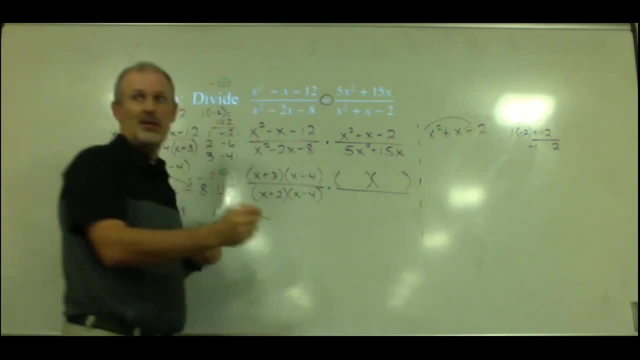 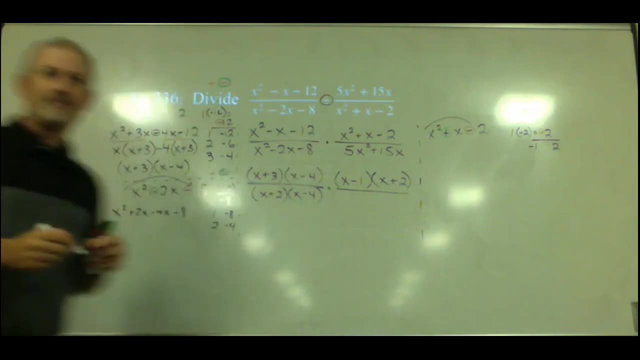 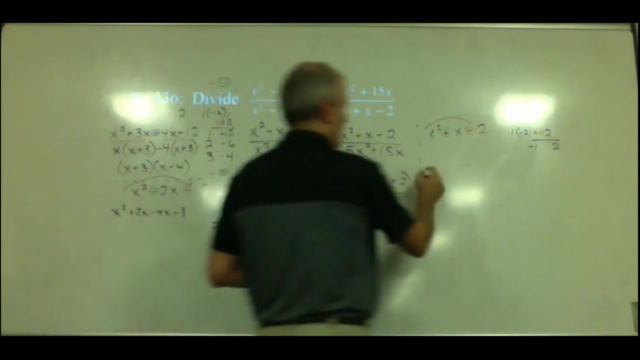 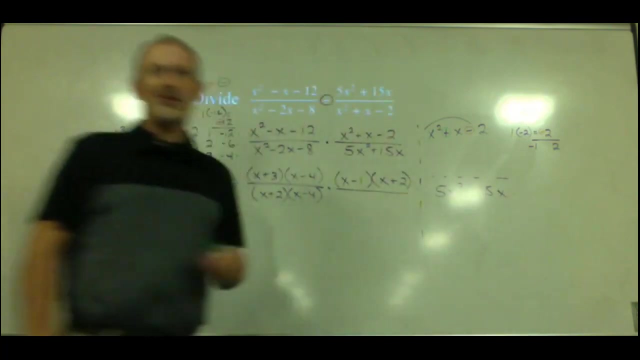 and we will have what As our two factors: X minus one and x plus two. Okay, and then we go to the last one: Five x squared plus 15 x. If you guys were rusty in your factoring, you're getting plenty of practice tonight. 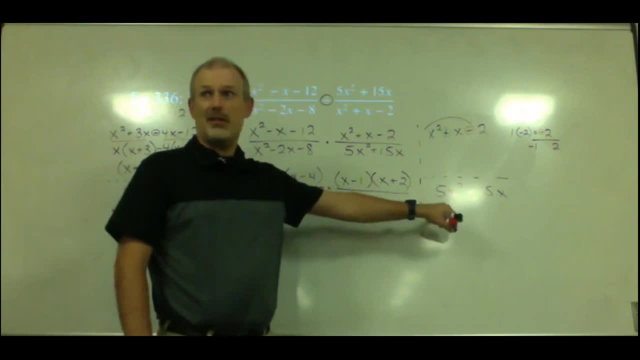 Now notice: this one is not just an x squared, It's an x squared Right, And it only has two terms. So first thought, really every time, and especially when it's not just an x squared is, is there a greatest common factor? 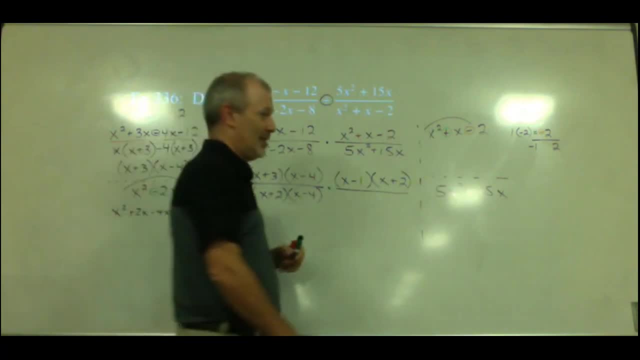 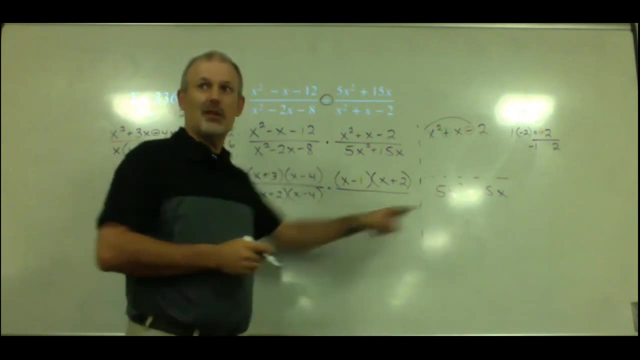 that we can factor out of everything. Why do you? oh, never mind, never mind. Okay, is there a greatest common factor here that we can use Five and notice they both have an x, So we can factor out a five and an x. 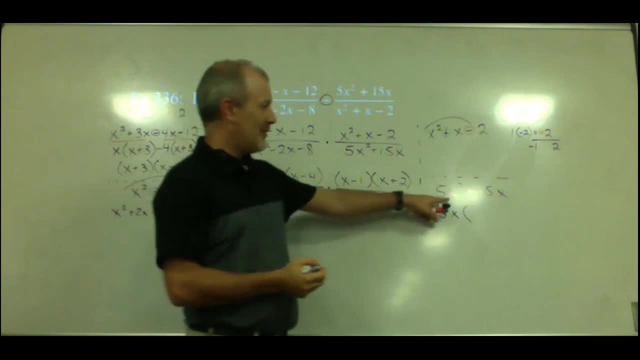 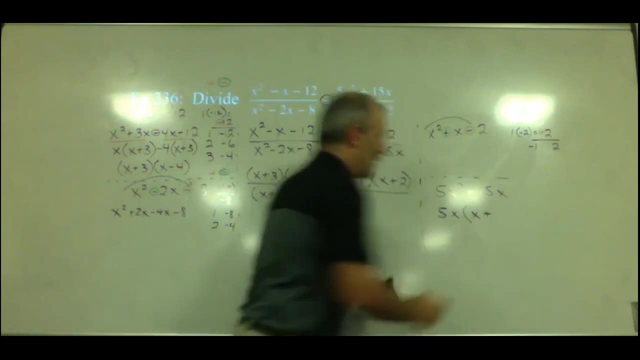 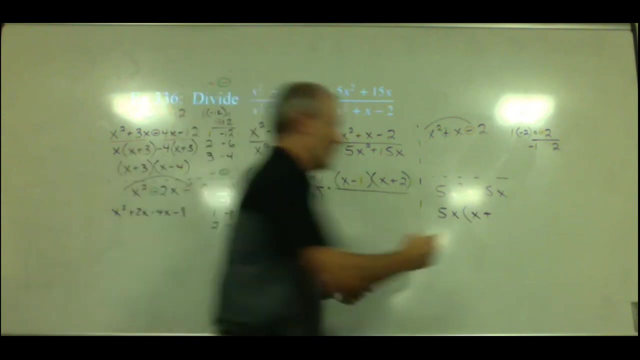 And if we factor out a five and an x from this first term, what's gonna be left there? An x. and then if we factor out a five and an x from the 15 x, what are we gonna have there? Because we are dividing, so it's gonna be three. 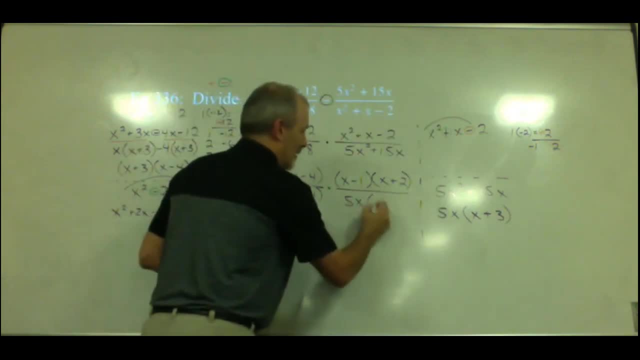 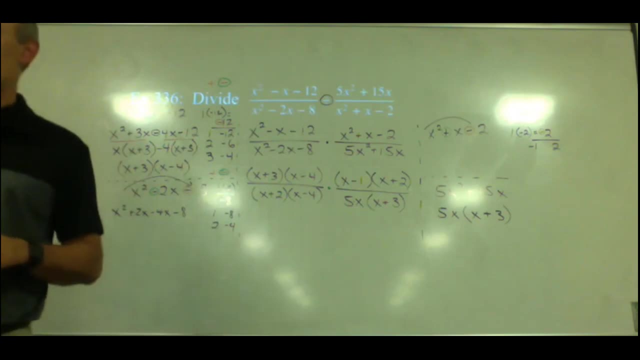 So that goes in down here. That's all we can do there. Now, one thing I do want to emphasize: this is five times x. Notice there's no plus sign or anything in between. Why? That's not the answer it. So we've got a 5 that we could possibly cancel. We've got an X that we 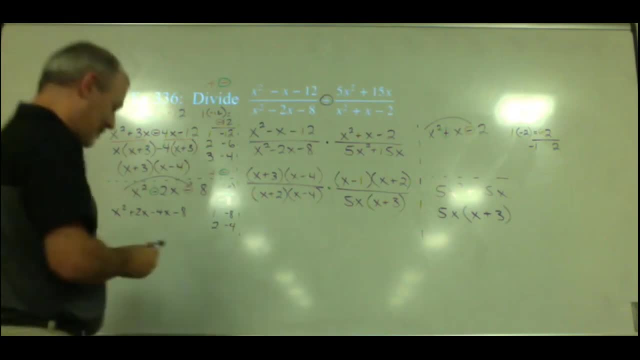 could possibly cancel. So now that we've got it all factored, do you see anything, hopefully that we can cancel? Remember it's got to be top to bottom: X plus 3.. Okay, X plus 3 cancels here and here. That's good, There's one gone- X minus 4.. 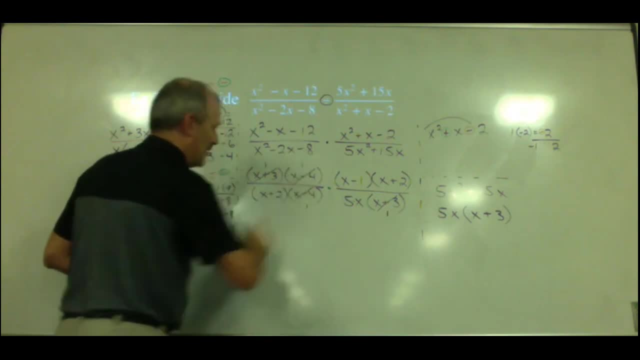 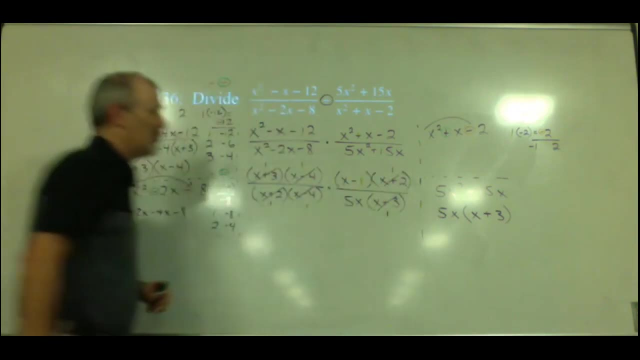 Okay, X- 4.. That's almost hiding right on top of each other, right? Okay, so those will cancel, like this: X plus 2.. Okay, and remember, you've got to cancel the whole parentheses at a time. They have to be identical the. 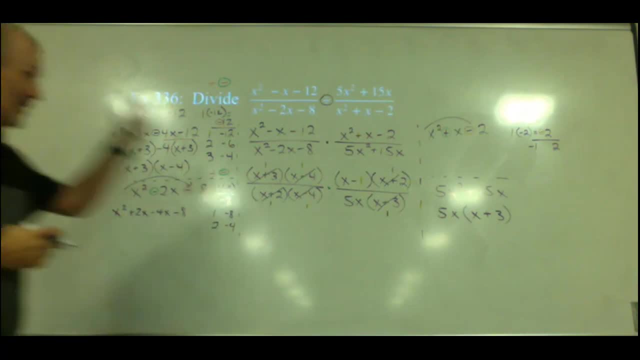 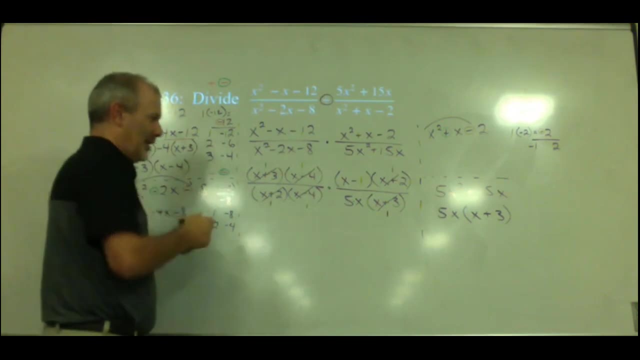 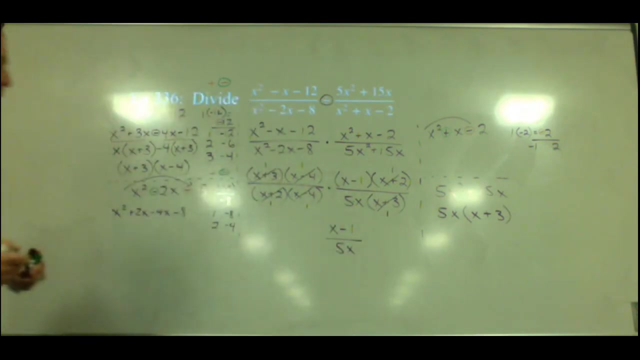 parentheses here. And that's it, because X minus 1, we don't have any X minus 1 down here, So our answer ends up being X minus 1 in the numerator and 5X in the numerator denominator. so you can see why we want to do that reducing and that canceling. 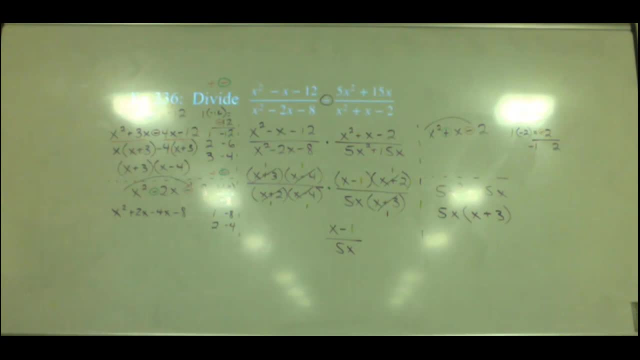 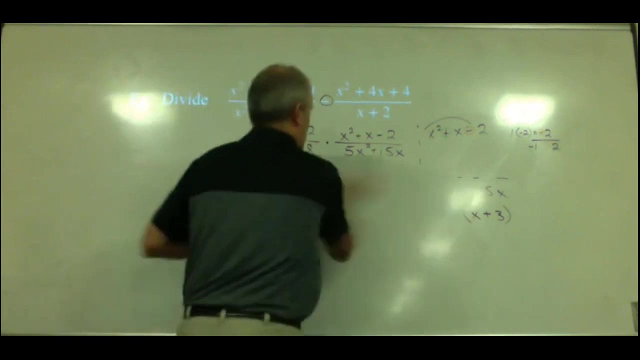 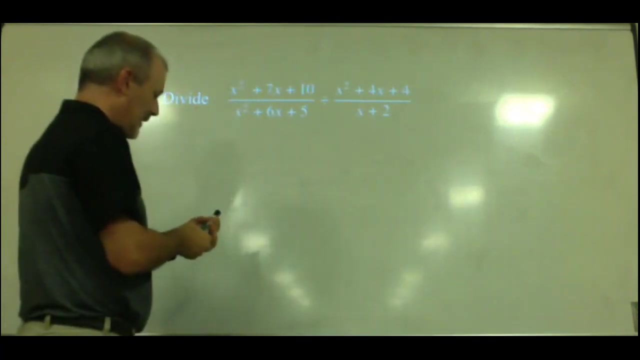 because then our answer gets a lot shorter. okay, that makes sense. and yes, it's a lot of factoring, I know. so you're gonna get your factoring practice. okay, before I erase that is everybody good, all right. so once again, hopefully we realize this is division and what do we? 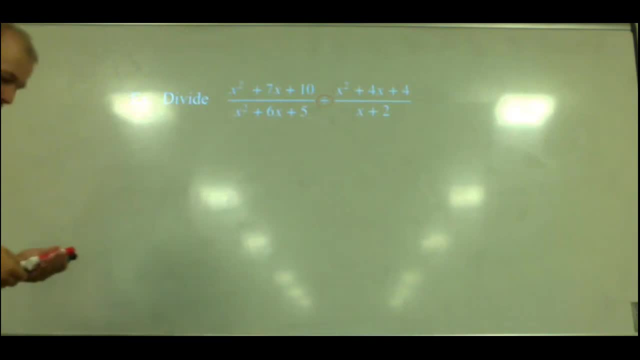 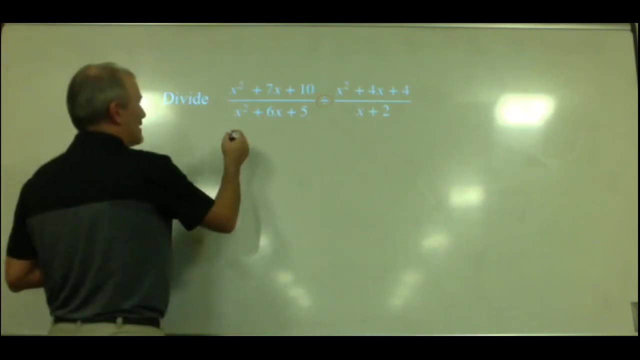 have to do anytime we see division? yeah, we're gonna switch it to multiple division. and what do we have to do anytime we see division? yeah, we're gonna switch it to multiple. fine, and we're gonna multiply by the reciprocal. reciprocal. all right, so the first one doesn't change: x squared plus 7x plus 10, then we have x squared plus. 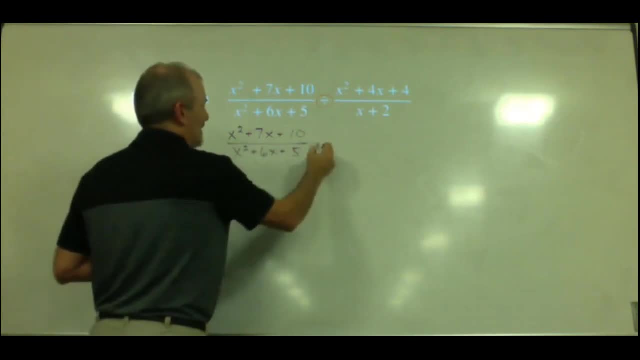 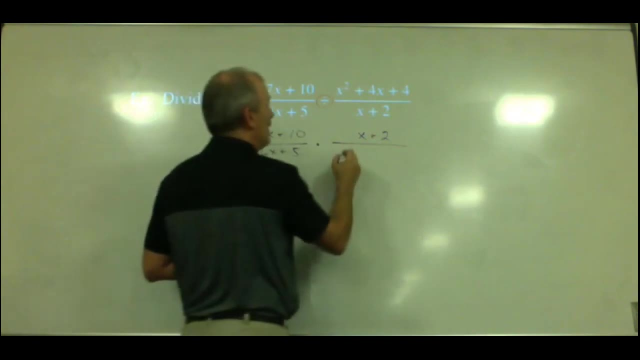 6x plus 5, and then it will become times, and now the x plus 2 is on the top. hey, we like this one because we don't have to factor anything right. x plus 2, and then x squared plus 4x plus 4 is on the bottom. 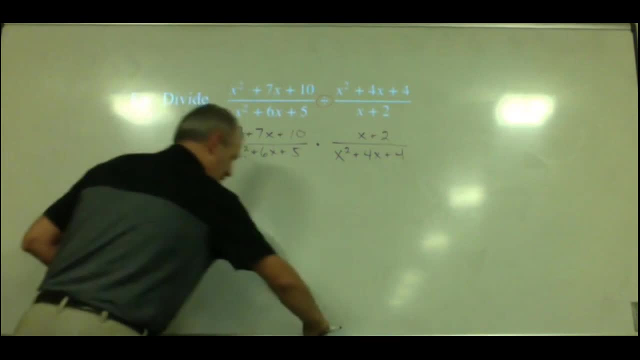 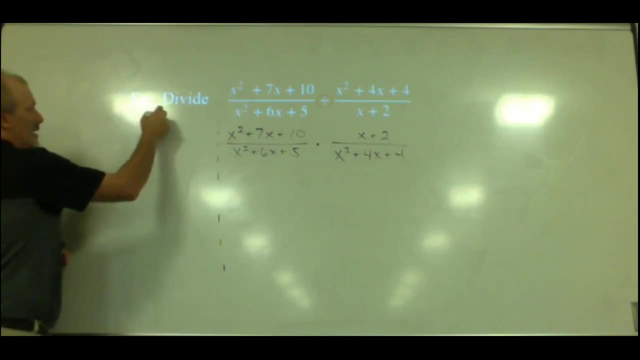 so now we are ready to factor. so again, let's do some of this work over here. the x squared plus 7x plus 10, we multiply this times this, we get 1 times 10 and that is 10, and since this is a positive 10, we haven't had this for a while at. 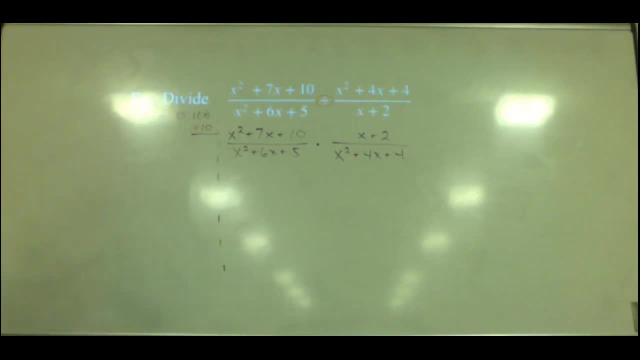 least not on the last question: what does that tell us about the signs of the numbers that we're looking for? yeah, they're both positive or they're both negative. so either both positive or both negative. and then, once we know that, we look over here and if they have the same sign and they add up to be a positive, 7. 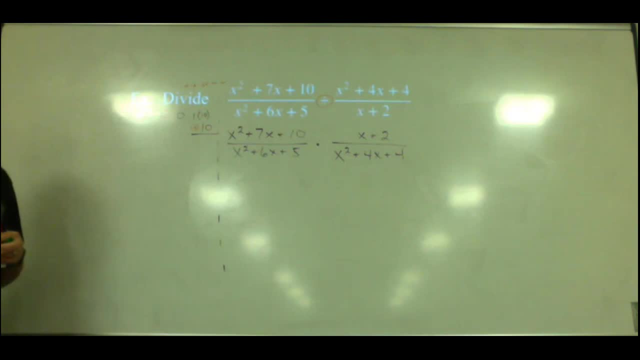 they would both have to be what. they would both have to be positive. so that's what we're looking for this time, is two positives for our factors of 10. so let's see if we can do this. first one: 1 and 10. does that add up to be 7? no, so we go to the next one: 2 and 5- yes, does that. 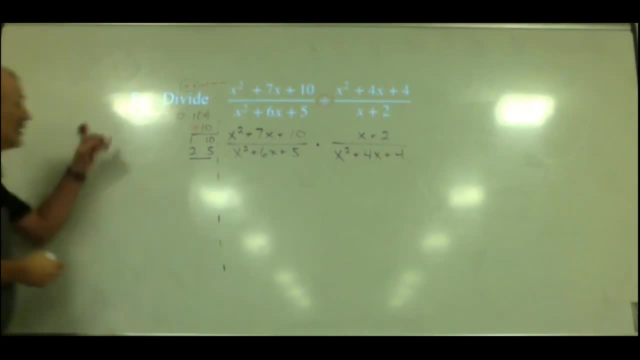 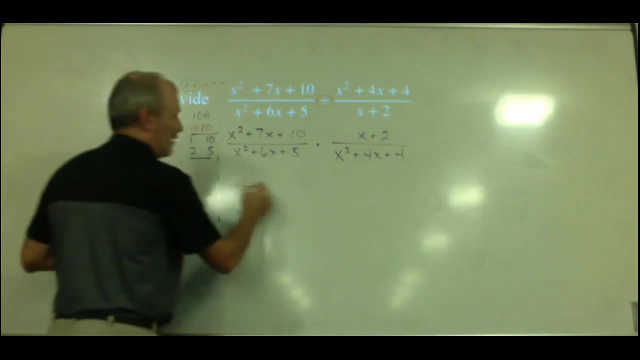 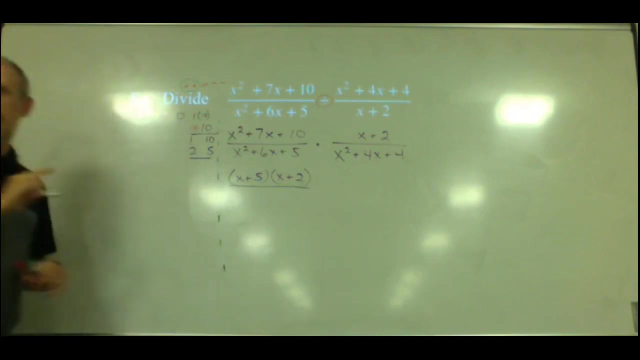 add up to be 7. yes, and again. right, we can use our shortcut. and because this is just an x squared, so what will the two factors be? x plus 5 and x plus 2, and again, the order that we write them in doesn't matter, as long as we 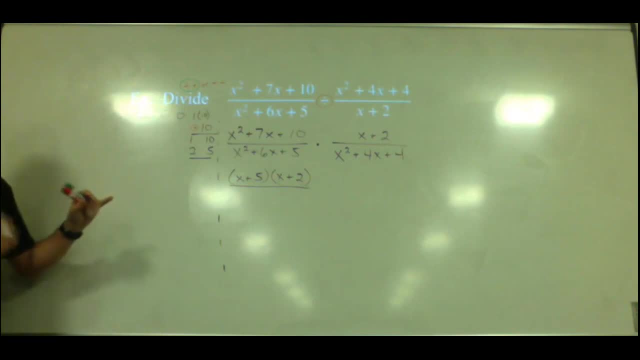 have the right factors. okay, is that? okay, that shortcut. do we understand what's going on? as long as this is an x squared, once we get these we can just put them into the parentheses. okay, let's go down here: x squared plus 6x plus 5. we multiply the 1 times the 5 and. 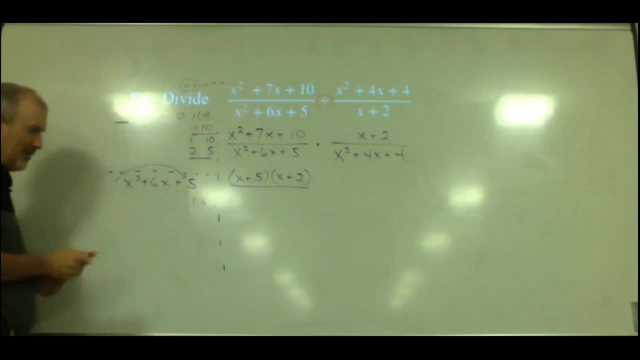 that is 5, and once again, this time it is a positive 5, and what does it mean to us that it is a, that it is a positive 5? they're both positive or they're both negative. once we know that we look over here at this. 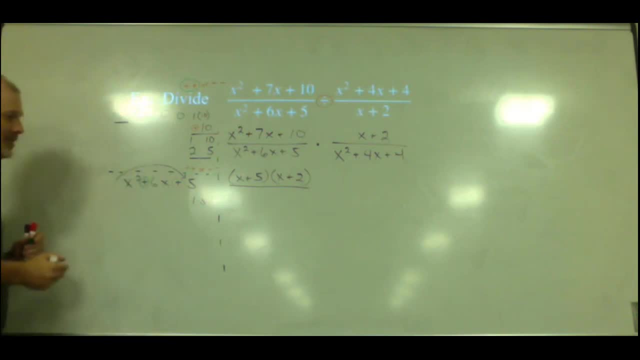 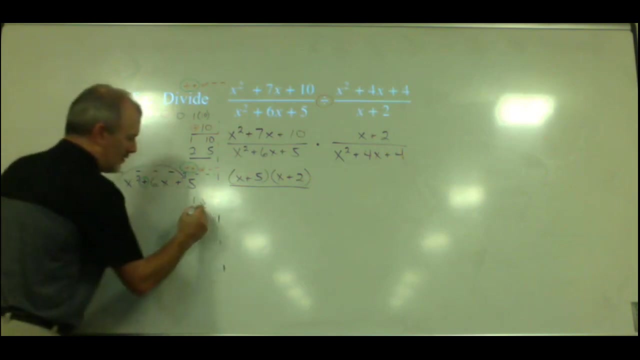 6, and since the 6 is a positive, we know what. they're both positive. so we're looking for two positive numbers that are multiples, that are factors of five. so five again is prime. the only options are one and bye. does that add up to be 6? 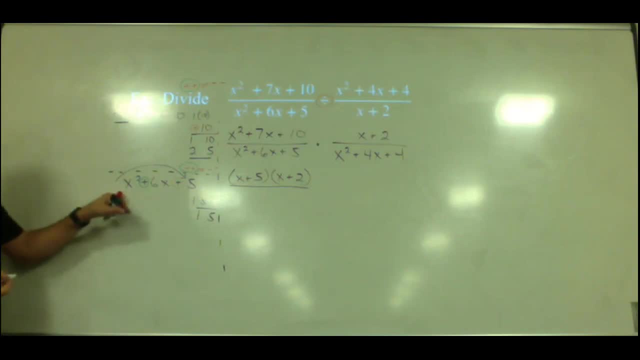 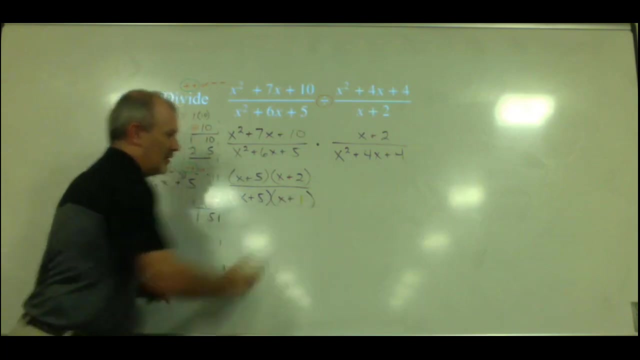 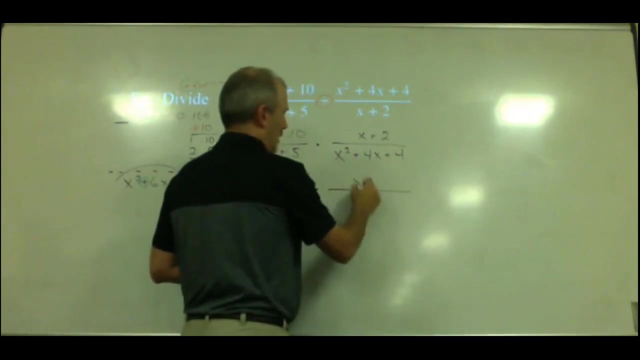 yeah, yes. so again, because this is just the next square, we can use our shortcut. and what will our two factors be if you know that those are the x plus 5 and x plus 1? x plus 5 and x plus 1, and remember, the x plus 2 we can't do anything with. 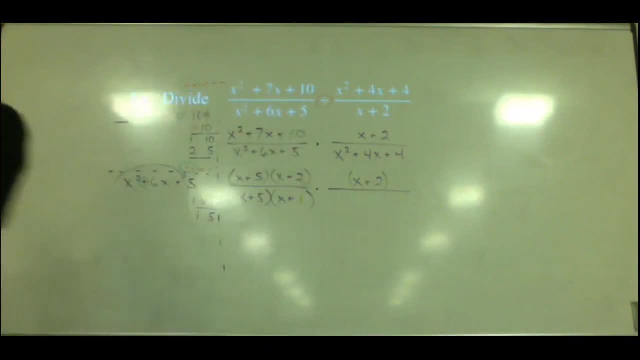 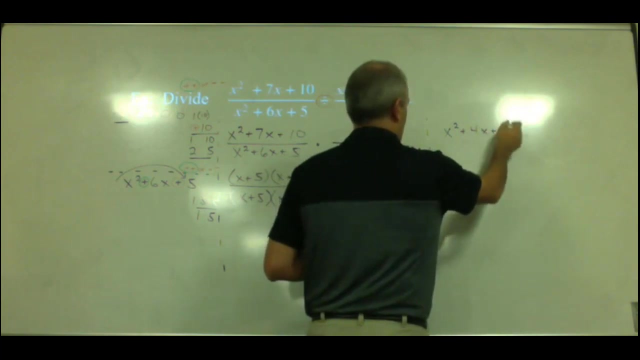 and I'm going to put parentheses around it just to emphasize that's a group. you have to cancel the whole thing if you're going to cancel something. and then we've got to factor this last one, the x squared plus 4x plus 4 boy, they're really putting us in a group here. 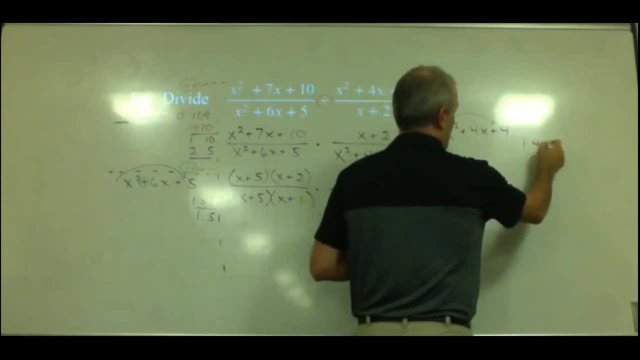 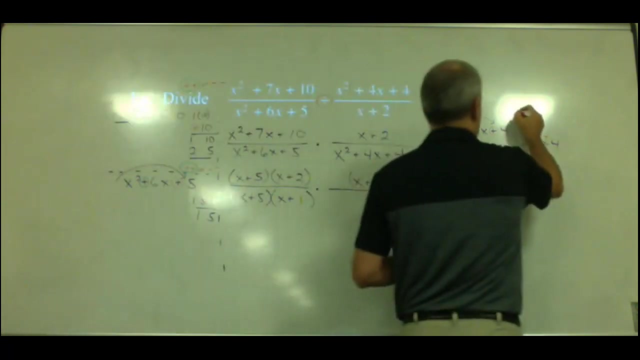 over and over again. so 1 times 4 is 4 and that is a positive 4. so what does that tell us? once again, they're both positive or they're both negative. they're the same sign, both positive or both negative. and then, once we know that, 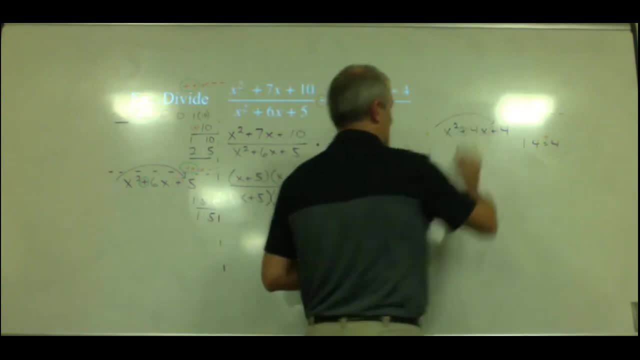 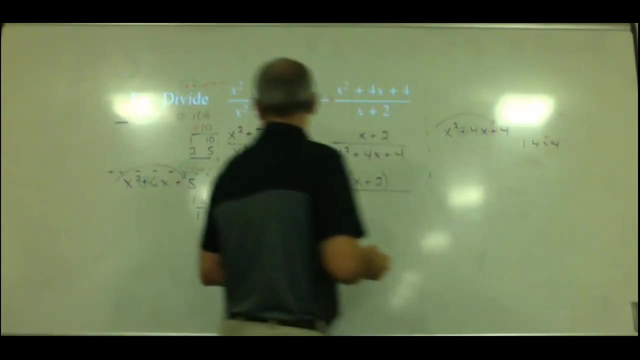 we can check this middle sign and since that's a positive, what does that tell us? they're both positive. kind of boring. all three of these that we were factoring were both the same and both positive. but you know we need practice on all these types. 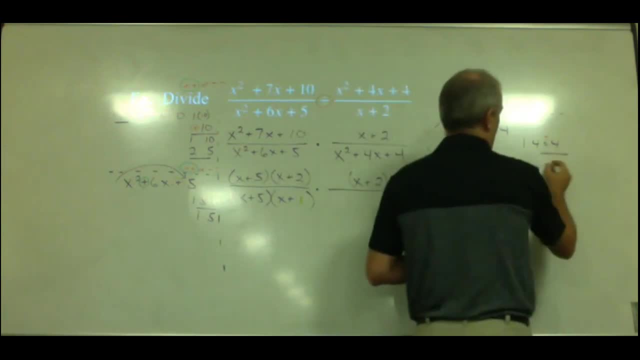 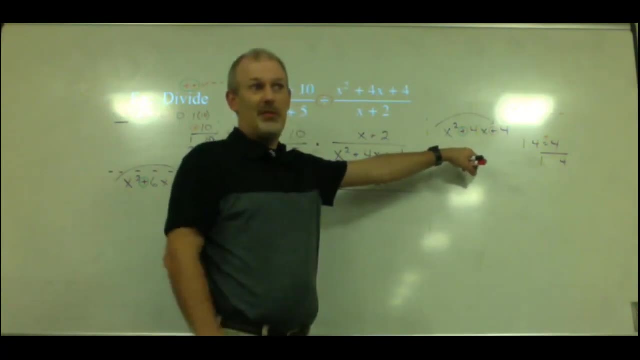 so both positive. 1 and 4 is our first option. does that add up to be 4?? now, be careful. does it add up to be 4?? because 1 and 4 are positive. because 1 and 4 are positive. because 1 and 4 are positive. 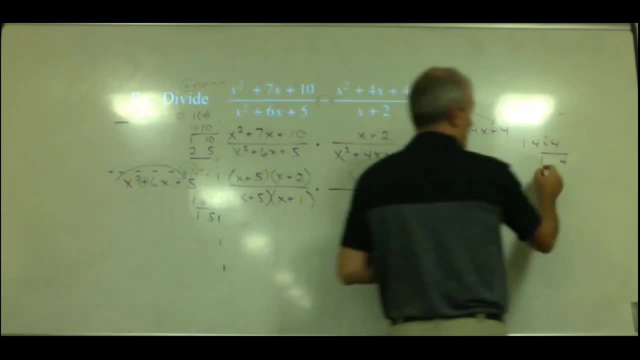 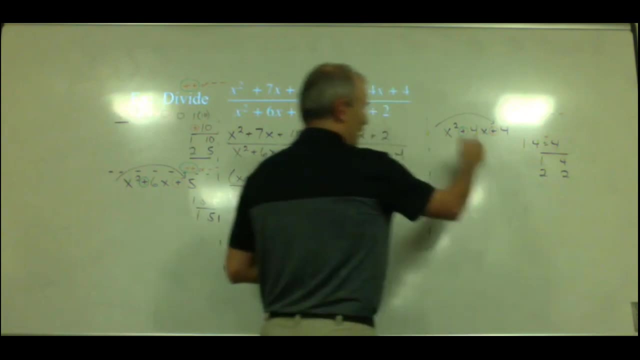 4 added is 5, so our next option will be 2 and 2. does that add up to be 4?? yeah, that's the one that works. so once we see that again, we are allowed to use our shortcut here, because it is just an x squared. 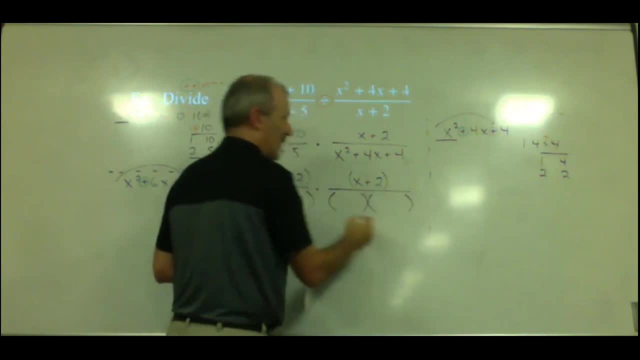 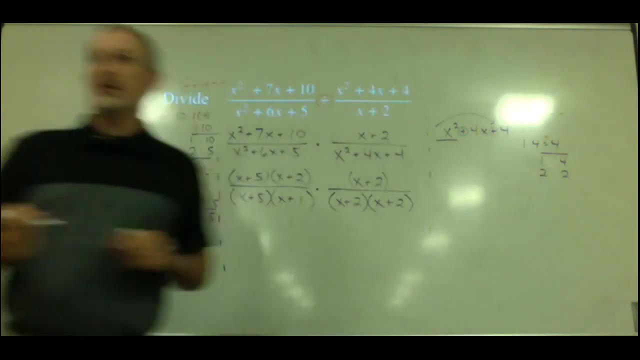 so our two factors will be what? x plus 2 and x plus 2? again, those are both positives, right? okay, so we are done with our factoring. so we are done with our factoring. once we're done with all of our factoring. 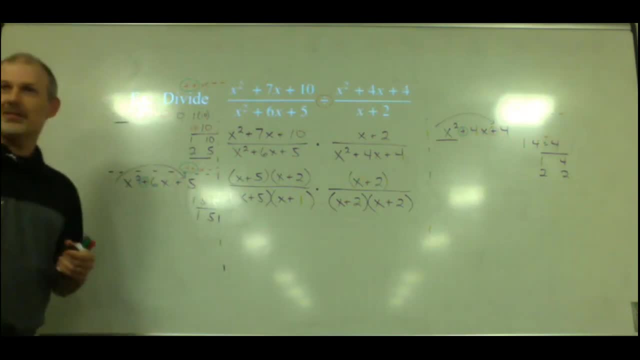 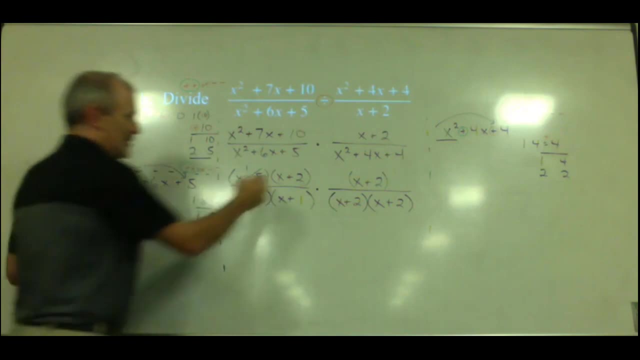 we look for things to cancel. what can we cancel? x plus 5. okay, x plus 5 and x plus 5. you lined them up there for us very nicely: x plus 2, x plus 2 and x plus 2 and x plus 2. 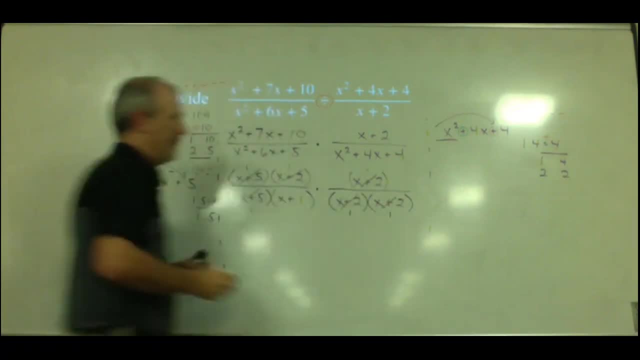 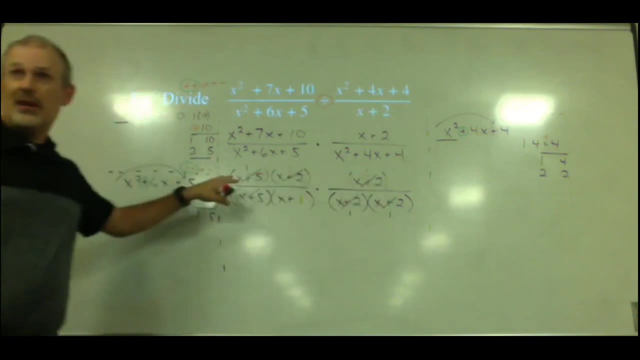 and another x plus 2 and x plus 2. okay. now here's where we have to be careful. we still have an x plus 1 on the bottom right and there's nothing else to cancel with on the top, correct? so here's what we have to be careful of. 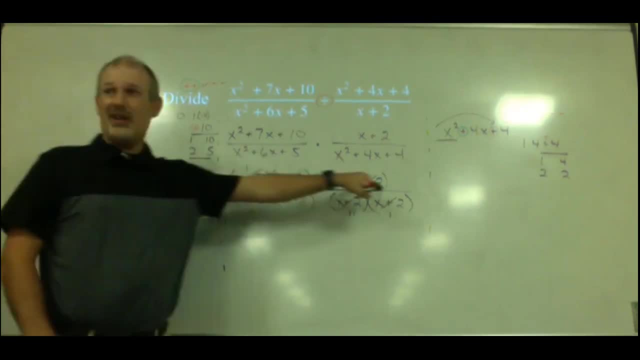 you'll notice every time we cancel with an x plus 2. you'll notice every time we cancel with an x plus 2, every time I write these, I'm putting in these ones and usually we just ignore them. right, and the reason we ignore them. 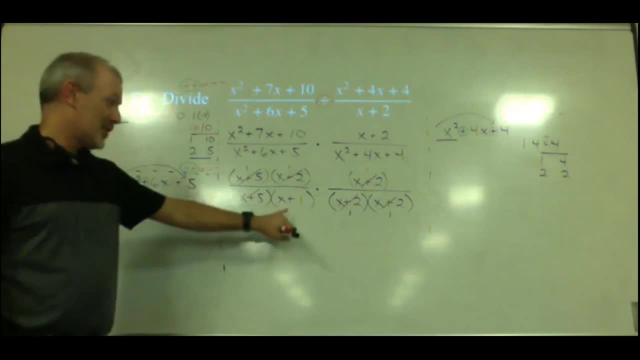 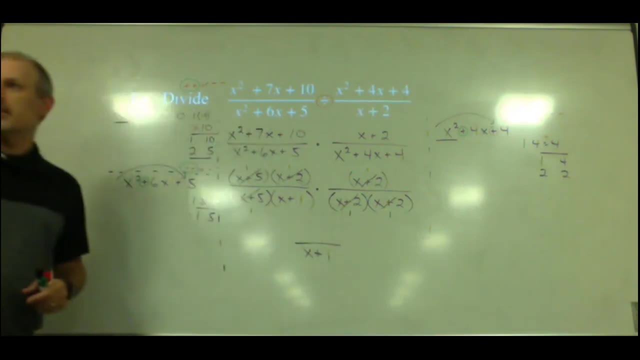 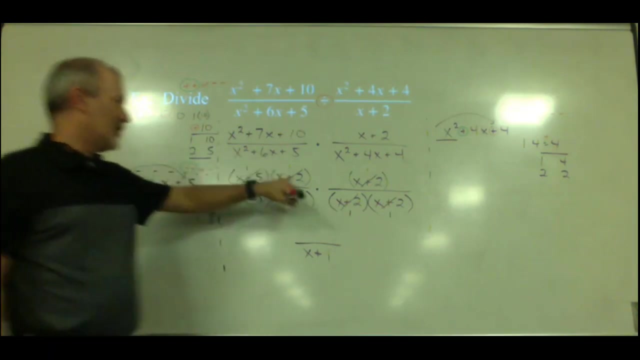 let's take a look at the bottom. 1 times x plus 1 times 1 times 1 is just x plus 1. right, because when you multiply by 1, nothing happens. but what do we have left on the top? 1 times 1 times 1. 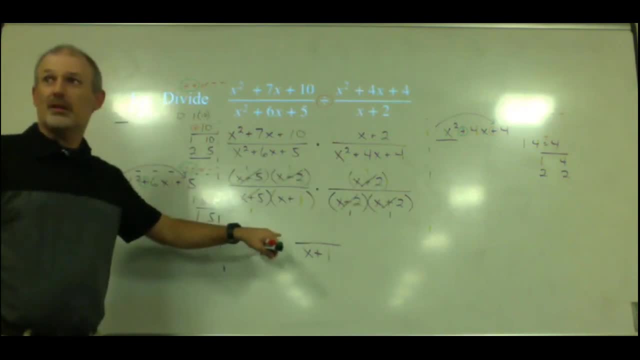 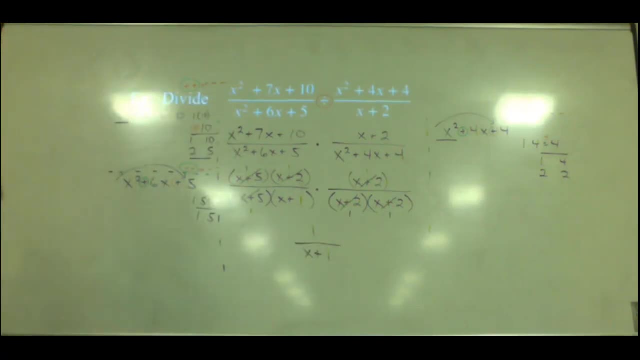 so what's on the top? 1? because you are multiplying. you're multiplying them by 1, and so we have 1 on the top and x plus 1 on the bottom. when you're multiplying, it's never going to like magically turn to a 0.